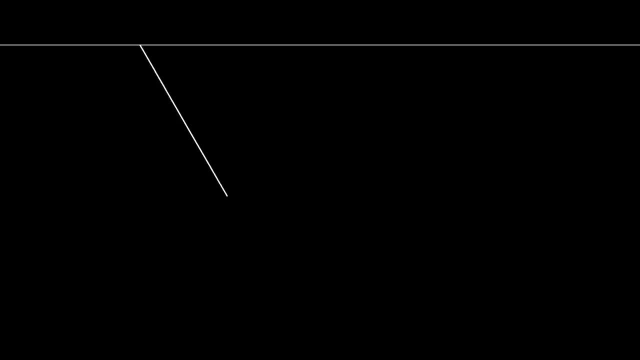 as a student was not in a calculus class but a physics class, We were studying a certain problem that had to do with the potential energy of a pendulum, and for that you need an expression for how high the weight of the pendulum is above its lowest point When you 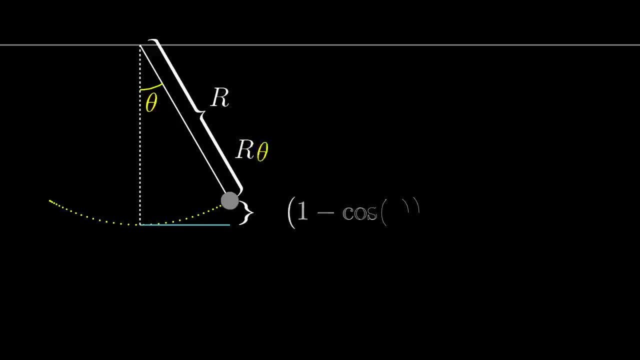 work that out, it comes out to be proportional to 1 minus the cosine of the angle between the pendulum and the vertical. The specifics of the problem we were trying to solve are beyond the point here, but what I'll say is that this cosine function made the problem. 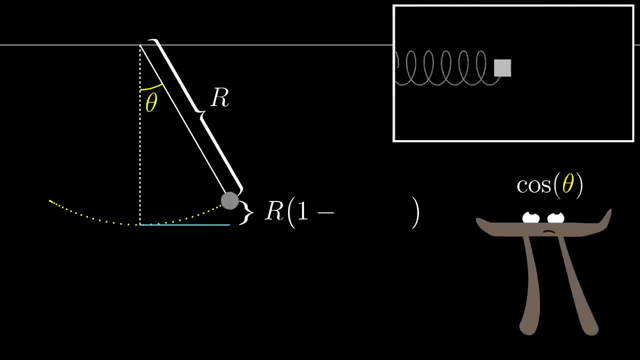 awkward and unwieldy and it made it less clear how pendulums relate to other oscillating phenomena. But if you approximate cosine of theta as 1 minus theta squared over 2,, of all things, everything just fell into place much more easily. If you've never seen anything. 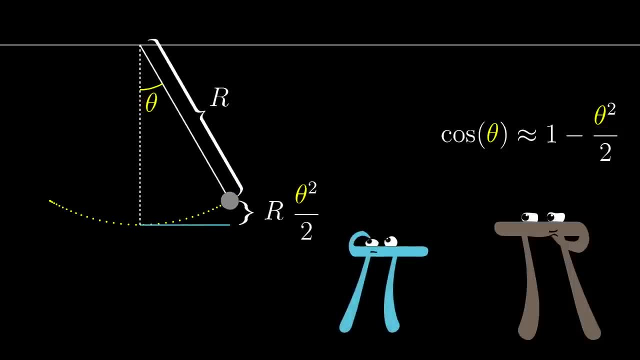 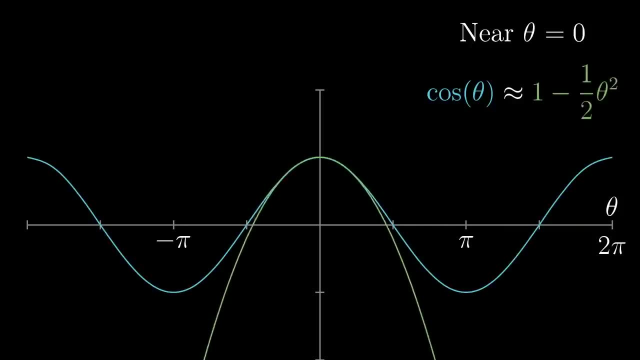 like this before. an approximation like that might seem completely out of left field. If you graph cosine of theta along with this function, 1 minus theta squared over 2, they do seem rather close to each other, at least for small angles near zero. but how would? 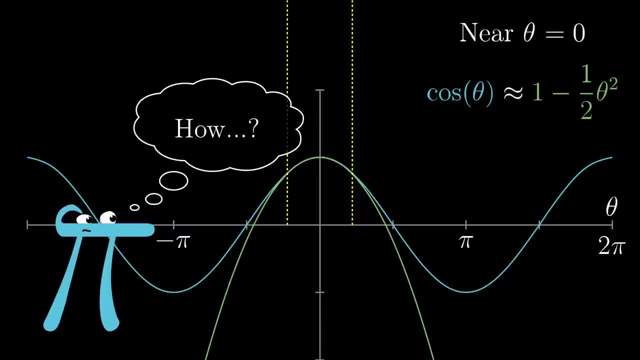 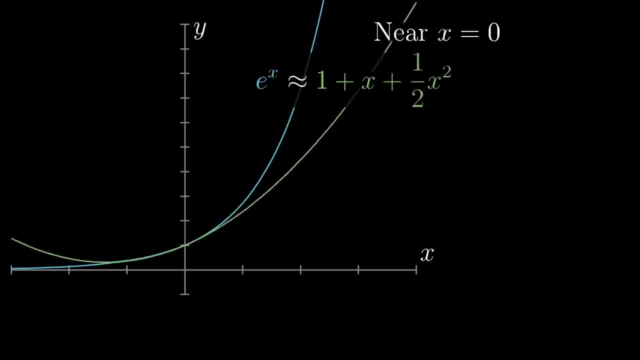 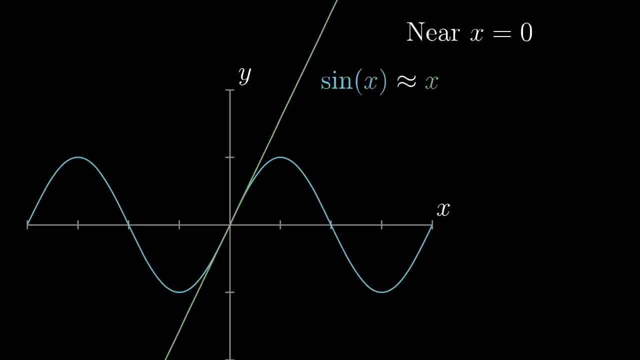 you even think to make this approximation and how would you find that particular quadratic? The study of Taylor series is largely about taking non-polynomial functions and finding polynomials that approximate them near some input. The motive here is that polynomials tend to be much easier to deal with than other functions. 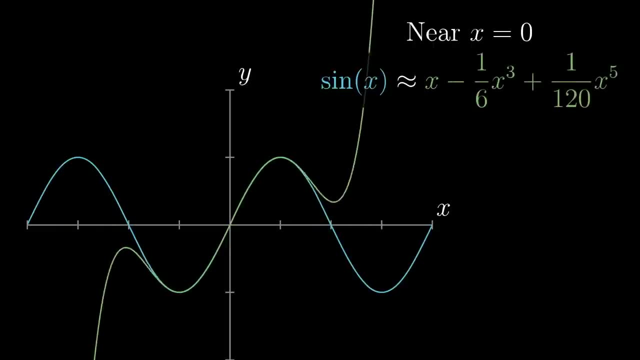 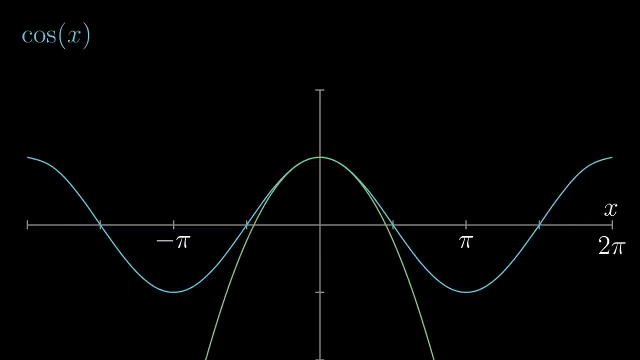 They're easier to compute, easier to take derivatives, easier to integrate, just all around more friendly. So let's take a look at that function, cosine of x, and really take a moment to think about how you might construct a quadratic approximation near x equals zero. That is among all of 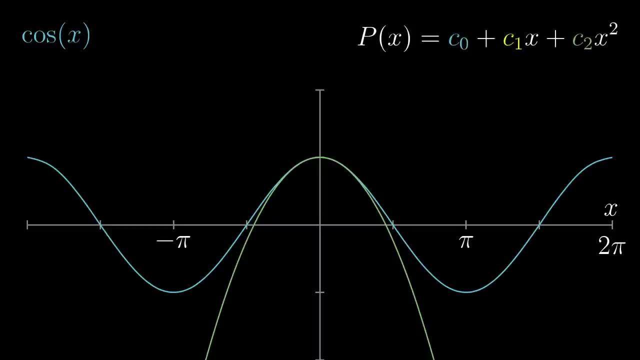 the possible polynomials that look like c0 plus c1 times x plus c2 times x, squared for some choice of these constants, c0,, c1, and c2.. Find the one that most resembles cosine of x near x equals zero. whose graph kind of spoons. 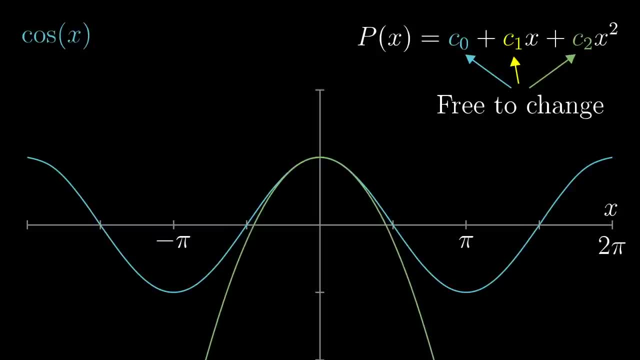 with the graph of cosine x at that point. First of all, at the input, 0, the value of cosine of x is 1, so if our approximation is going to be any good at all, it should also equal 1. at the input, x equals 0.. Plugging. 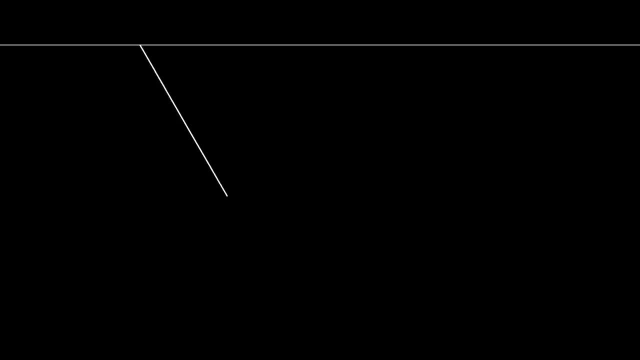 as a student was not in a calculus class but a physics class, We were studying a certain problem that had to do with the potential energy of a pendulum, and for that you need an expression for how high the weight of the pendulum is above its lowest point When you 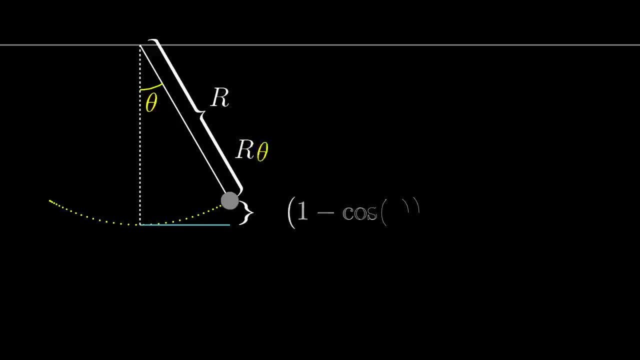 work that out, it comes out to be proportional to 1 minus the cosine of the angle between the pendulum and the vertical. The specifics of the problem we were trying to solve are beyond the point here, but what I'll say is that this cosine function made the problem. 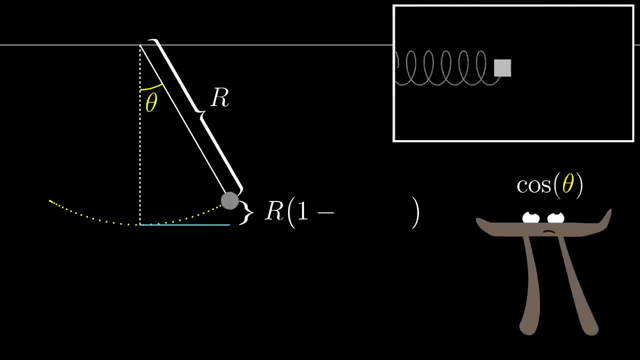 awkward and unwieldy and it made it less clear how pendulums relate to other oscillating phenomena. But if you approximate cosine of theta as 1 minus theta squared over 2,, of all things, everything just fell into place much more easily. If you've never seen anything. 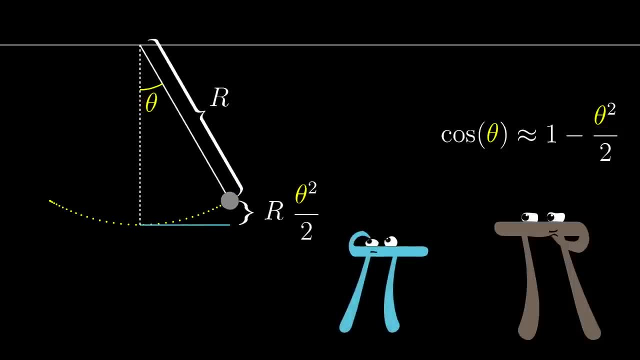 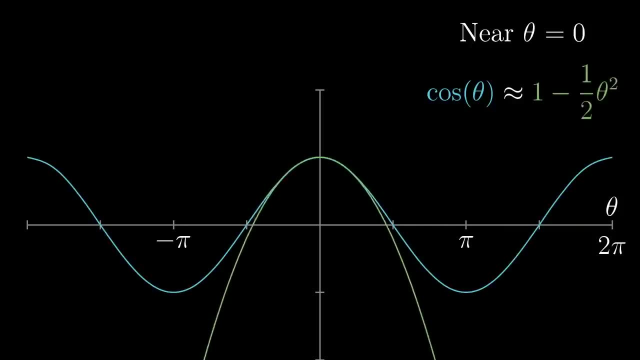 like this before. an approximation like that might seem completely out of left field. If you graph cosine of theta along with this function, 1 minus theta squared over 2, they do seem rather close to each other, at least for small angles near zero. but how would? 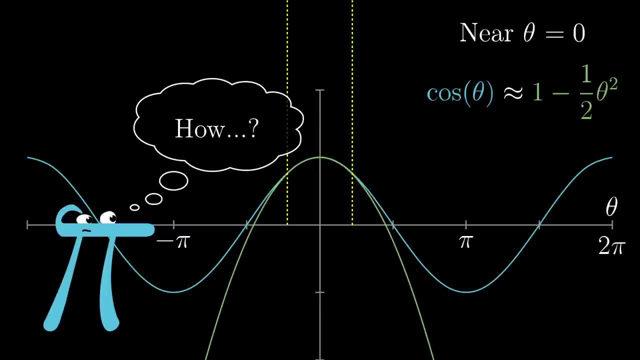 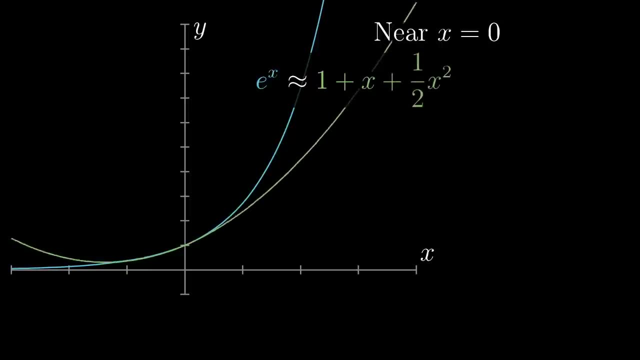 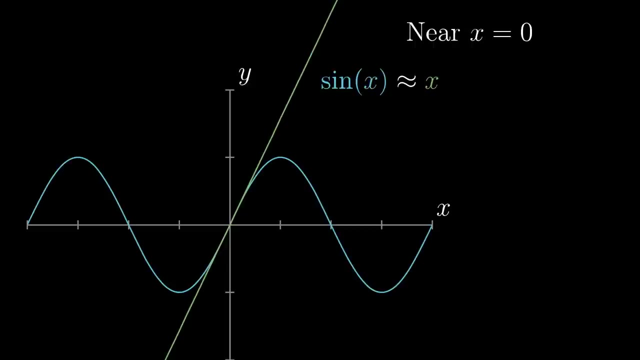 you even think to make this approximation and how would you find that particular quadratic? The study of Taylor series is largely about taking non-polynomial functions and finding polynomials that approximate them near some input. The motive here is that polynomials are easier to compute, easier to take derivatives and easier to integrate, just all around. 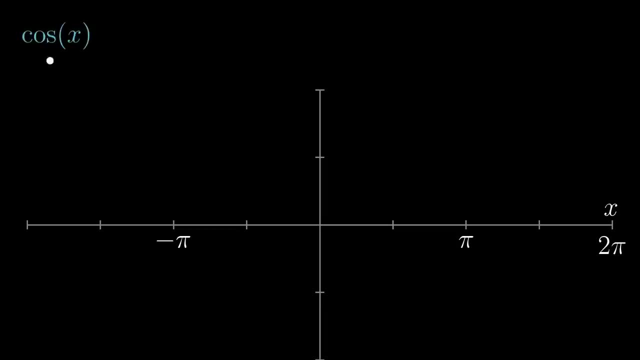 more friendly. So let's take a look at that function, cosine of x, and really take a moment to think about how you might construct a quadratic approximation near x equals zero. That is among all of the possible polynomials that look like c0 plus c1 times x plus c2 times x squared for. 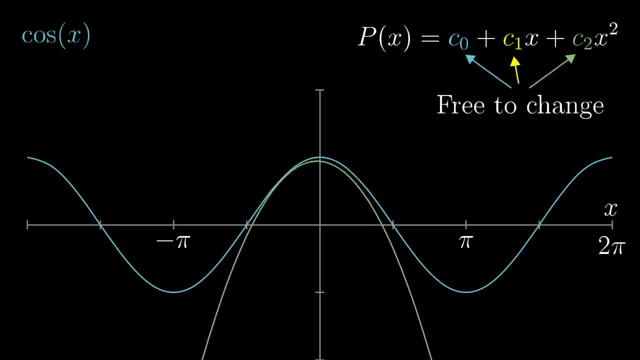 some choice of these constants, c0,, c1, and c2.. Find the one that most resembles cosine of x near. x equals zero, whose graph kind of spoons with the graph of cosine x. at that point, First of all, at the input zero, the value of cosine of x is 1, so if our approximation 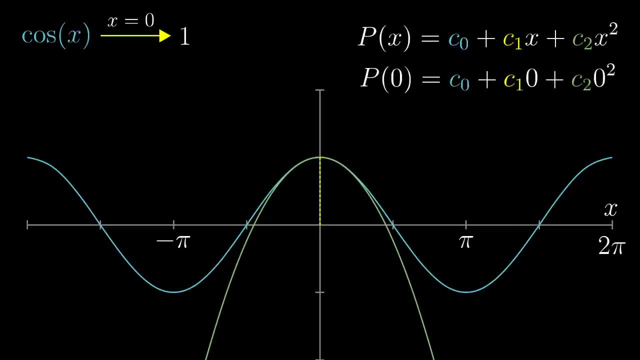 is going to be any good at all, it should also equal 1 at the input. x equals zero. Plugging in zero just results in whatever c0 is, so we can set that equal to 1.. This leaves us free to choose constants c1 and c2 to make this approximation as good as we can. but 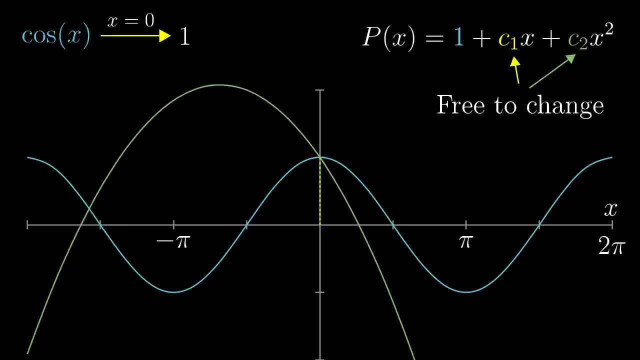 nothing we do with them is going to change the fact that the polynomial equals 1 at x equals zero. Now it would also be good if our approximation had the same tangent slope as cosine x at this point of interest. Otherwise the approximation drifts away from the cosine graph much faster. 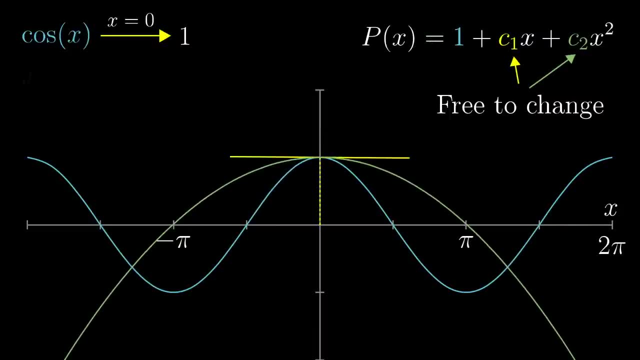 than it needs to. The derivative of cosine is negative sine and at x equals zero. that equals zero. On the other hand, when you work out the derivative of our quadratic, you get c1 plus 2 times c2 times x. At x equals zero. this just equals whatever we choose for c1. So 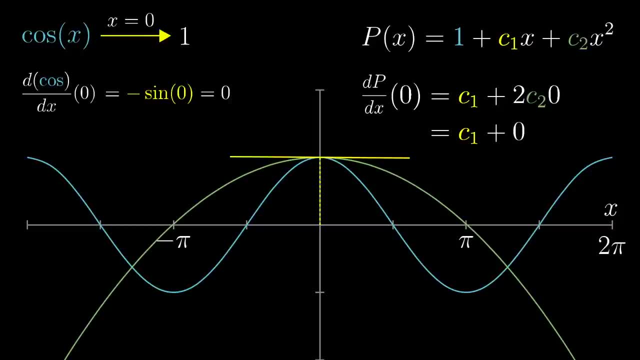 this constant c1, has complete control over the derivative of our approximation around. x equals zero. Setting it equal to zero ensures that our approximation also has a flat tangent line at this point. This gives us freedom to change c2.. Even so, the value and slope of our polynomial are: 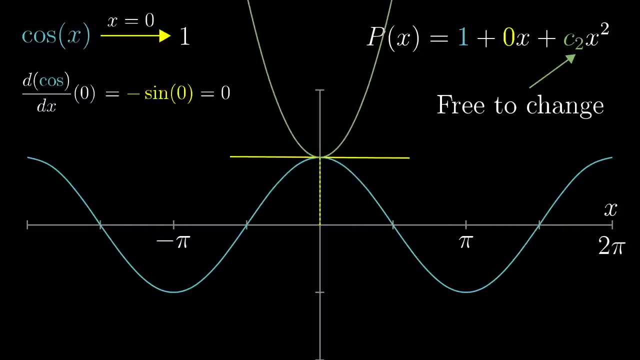 locked in place to match the value of cosine for each of the two. The final thing to take advantage of is the cosine graph curves downward above x equals zero, giving us a negative second derivative. Or, in other words, even though the rate of change is zero at that point, the rate itself is decreasing around that point. Specifically, 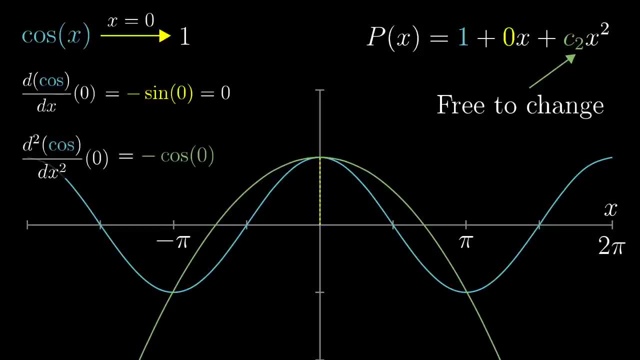 its derivative is negative sine of x. its second derivative is negative cosine of x, and at x equals 0, that equals negative 1.. Now, in the same way that we wanted the derivative of our approximation to match that of the cosine, so that their values wouldn't drift, 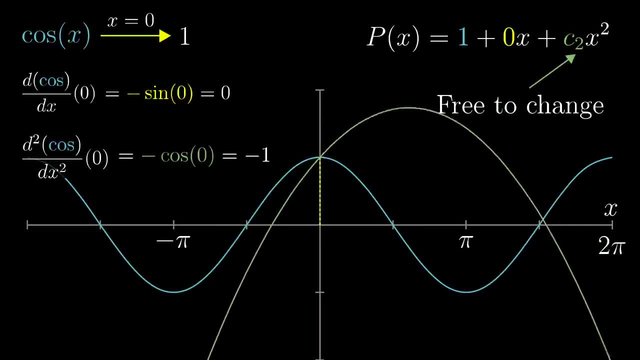 apart needlessly quickly. making sure that their second derivatives match will ensure that they curve at the same rate that the slope of our polynomial doesn't drift away from the slope of cosine x any more quickly than it needs to. Pulling up the same derivative we had before and then taking its derivative, we see that. 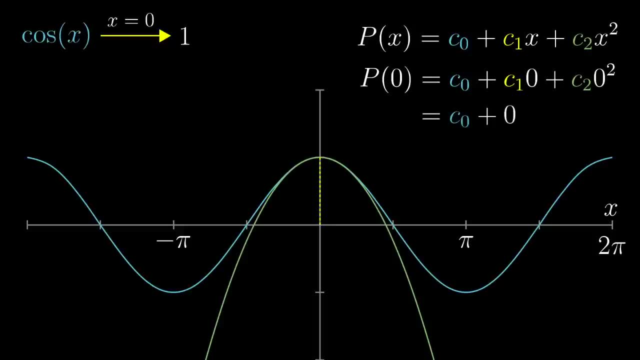 in 0 just results in whatever c0 is, so we can set that equal to 1.. This leaves us free to choose constants c1 and c2 to make this approximation as good as we can, but nothing we do with them is going to change the fact that the polynomial equals 1 at x equals 0. 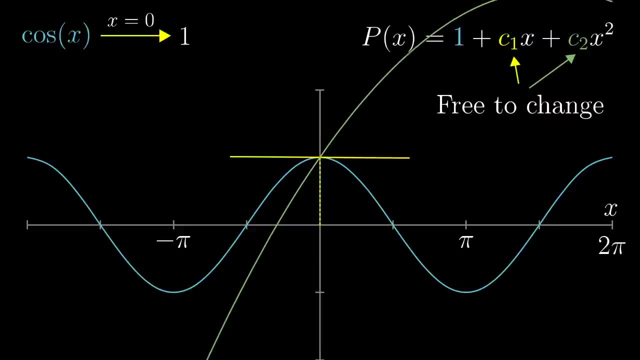 Now it would also be good if our approximation had the same tangent slope as cosine x at this point of interest. Otherwise the approximation drifts away from the cosine graph much faster than it needs to. The derivative of cosine is negative sine and at x equals 0, that 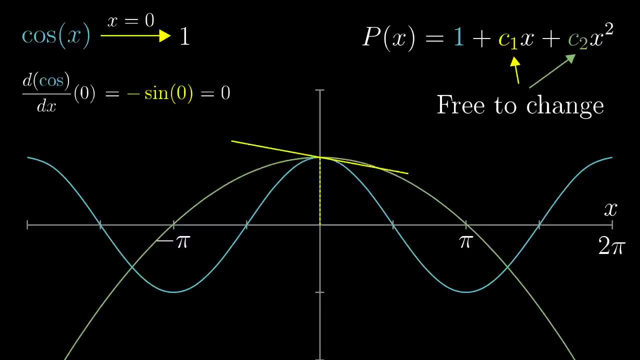 equals 0.. On the other hand, when you work out the derivative of our quadratic, you get c1 plus 2 times c2 times x At x equals 0, this just equals whatever we choose for c1. So this constant c1 has complete control over the derivative of our approximation around x equals. 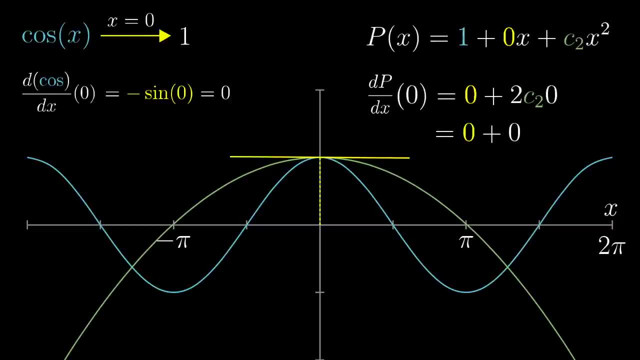 0. Setting it equal to 0 ensures that our approximation also has a flat tangent line at this point. This leaves us free to change c2.. But the value and the slope of our polynomial, at x equals 0, are locked in place to match that of cosine. 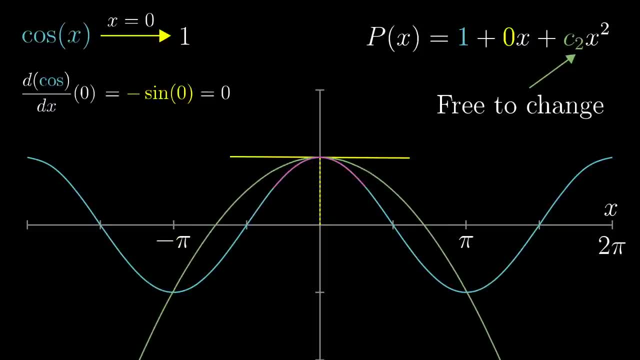 The final thing to take advantage of is that the cosine graph curves downward above. x equals 0. It has a negative second derivative, Or, in other words, even though the rate of change is 0 at that point, the rate of change itself is decreasing around that point. Specifically, 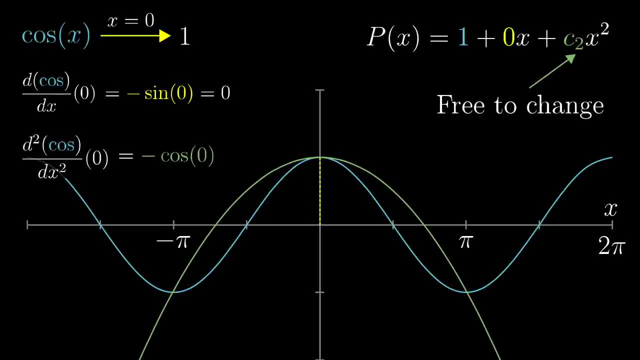 Since its derivative is negative, sine of x, its second derivative is negative cosine of x, and at x equals 0, that equals negative 1.. Now, in the same way that we wanted the derivative of our approximation to match that of the cosine, so that their values wouldn't drift apart needlessly, quickly making sure that 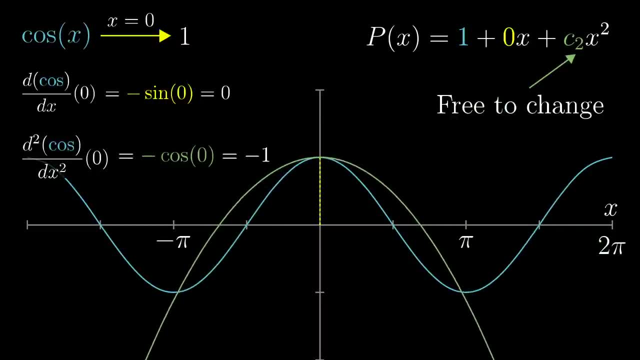 their second derivatives match will ensure that they curve at the same rate that the slope of our polynomial doesn't drift away from the slope of cosine x any more quickly than it needs to. Pulling up the same derivative we had before and then taking its derivative, we see that 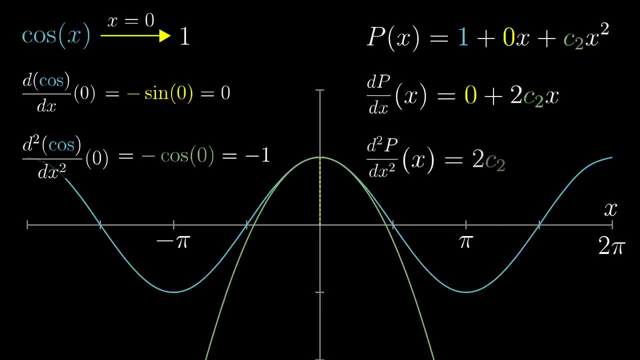 the second derivative of this polynomial is exactly 2 times c2.. So to make sure that this second derivative also equals negative 1 at x equals 0,, 2 times c2 has to be negative 1, meaning c2 itself should be negative 1 half And this gives us the approximation. 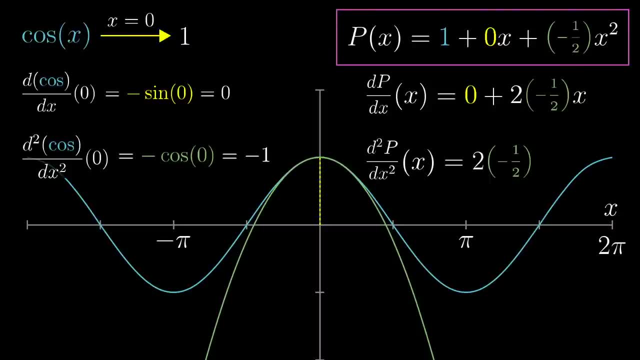 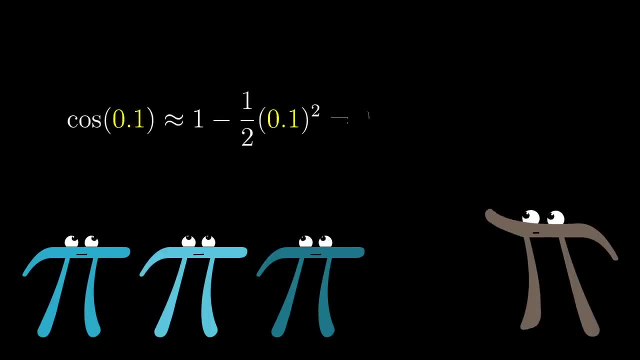 1 plus 0.. 0x minus 1 half x squared. And to get a feel for how good it is, if you estimate, say, cosine of 0.1 using this polynomial, you'd estimate it to be 0.995.. And this is the true value of cosine of 0.1.. It's a really 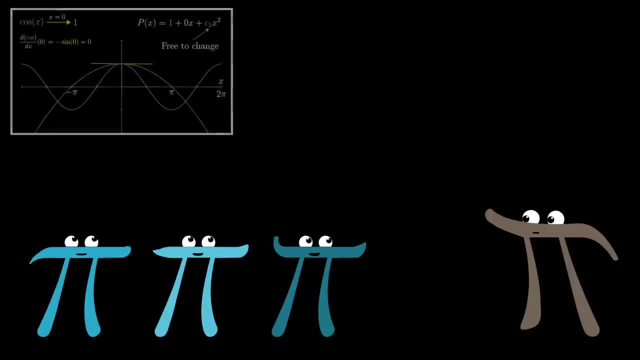 good approximation. Take a moment to reflect on what just happened. You had three degrees of freedom with this quadratic approximation: the constants c0,, c1, and c2.. c0 was responsible for making sure that the output of the approximation matches that of 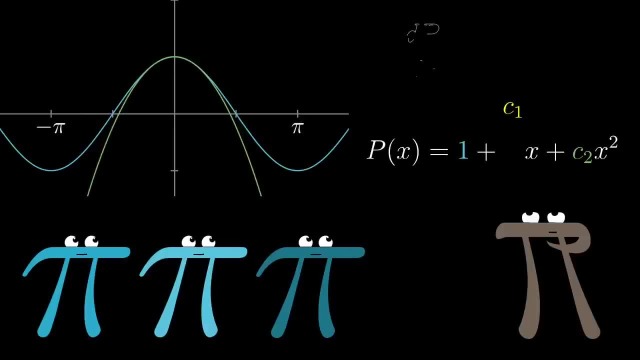 cosine x at x equals 0,. c1 was in charge of making sure that the derivatives match at that point and c2 was responsible for making sure that the second derivatives match up. This ensures that the way your approximation changes as you move away from x equals 0,. 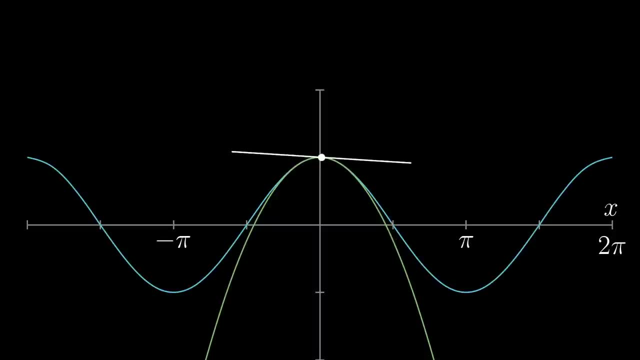 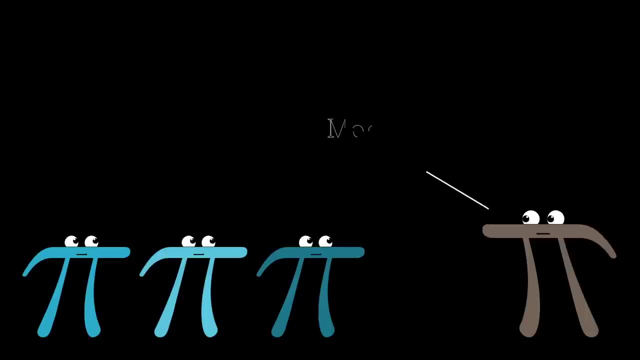 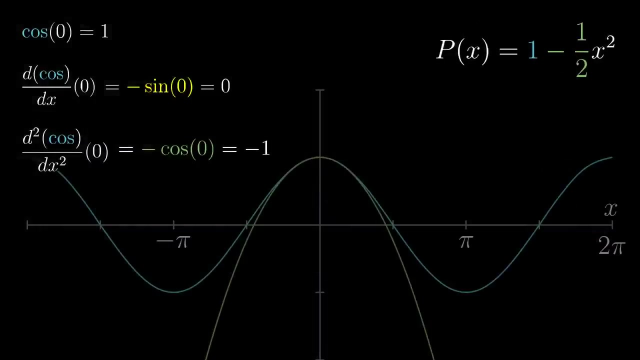 and the way that the rate of change itself changes is as similar as possible to the behavior of cosine x. given the amount of control that you have, You could give yourself more control by allowing more terms in your polynomial and matching higher order derivatives. For example, let's say you added on the term c3 times x cubed. 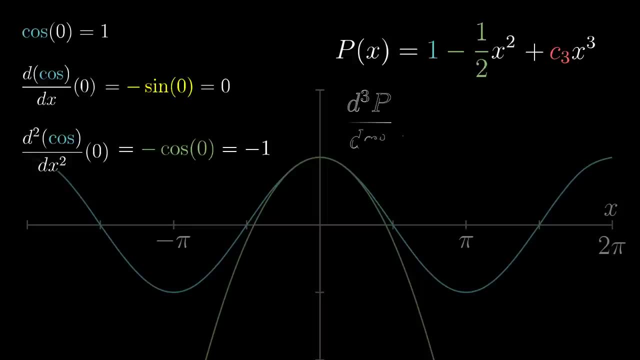 for some constant c3.. Well, in that case, if you take the third derivative of a cubic polynomial, anything that's quadratic or smaller goes to 0.. And as for that last term, after three iterations of the power rule, you'd have 0.995. 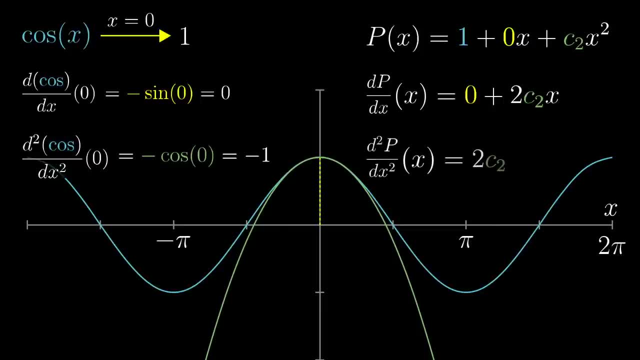 the second derivative of this polynomial is exactly 2 times c2.. So to make sure that this second derivative also equals negative 1 at x equals 0,, 2 times c2 has to be negative 1, meaning c2 itself should be negative 1 half. 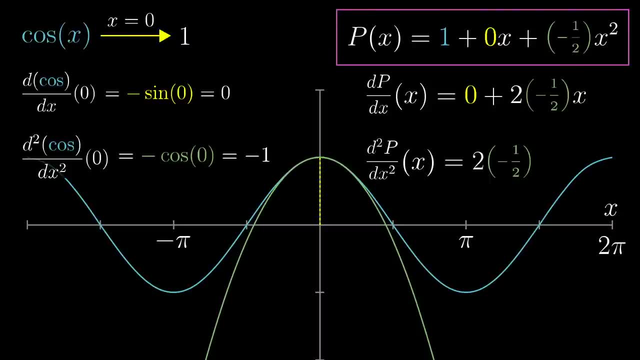 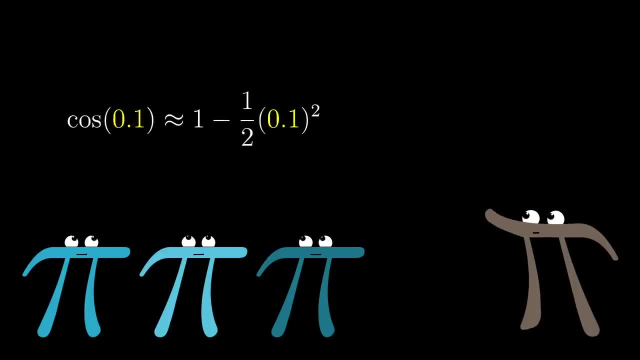 And this gives us the following derivative: This gives us the approximation 1 plus 0x minus 1 half x squared. And to get a feel for how good it is, if you estimate, say, cosine of 0.1 using this polynomial: 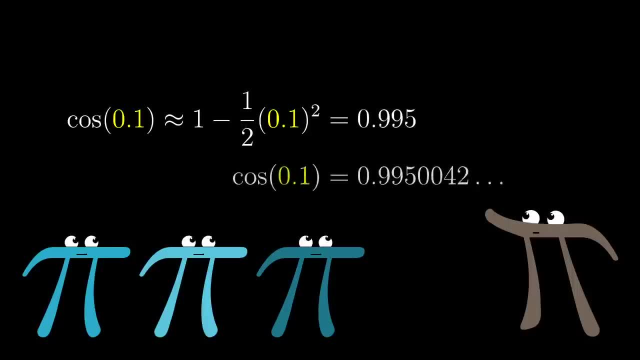 you'd estimate it to be 0.995.. And this is the true value of cosine of 0.1. It's a really good approximation. Take a moment to reflect on what just happened. You had 3 degrees of freedom with this quadratic approximation. 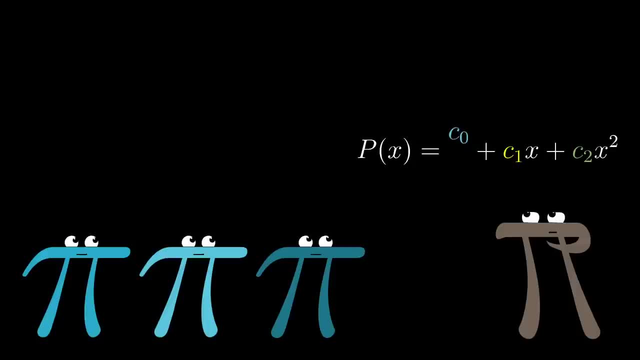 The constant c0,, c1, and c2.. c0 was responsible for making sure that the output of the approximation matches that of cosine x, at x equals 0. c1 was in charge of making sure that the derivatives match at that point. 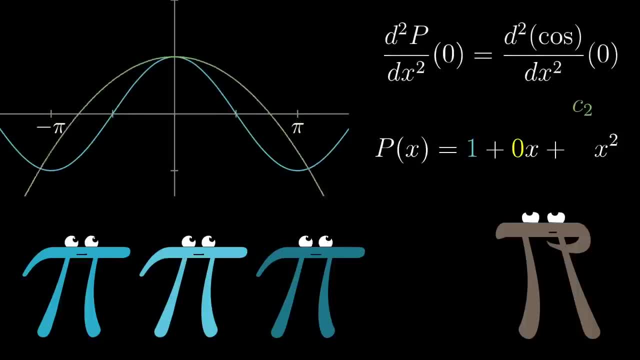 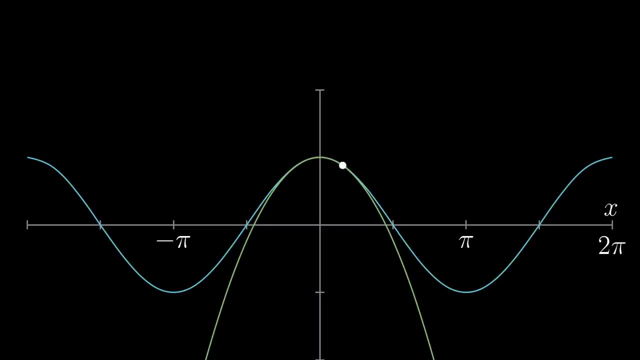 And c2 was responsible for making sure that the second derivative matches. This ensures that the way your approximation changes as you move away from x equals 0, and the way that the rate of change itself moves away from x equals 0, is the same as. 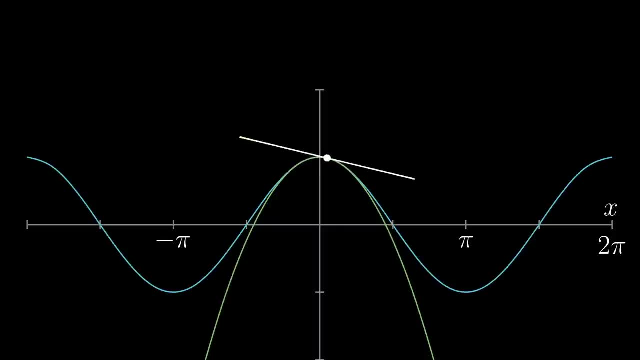 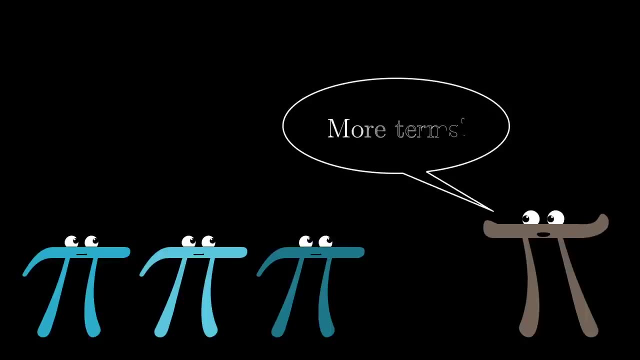 the way that the rate of change itself moves away from x equals 0.. The way that the rate of change itself changes is as similar as possible to the behavior of cosine x. given the amount of control that you have, You could give yourself more control by allowing more terms in your polynomial and matching. 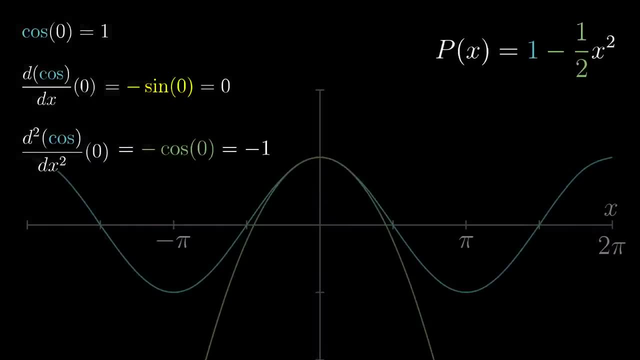 higher order derivatives. For example, let's say you added on the term c3 times x, cubed for some constant c3. Well, in that case, if you take the third derivative of a cubic polynomial, anything that's quadratic or smaller goes to 0.. 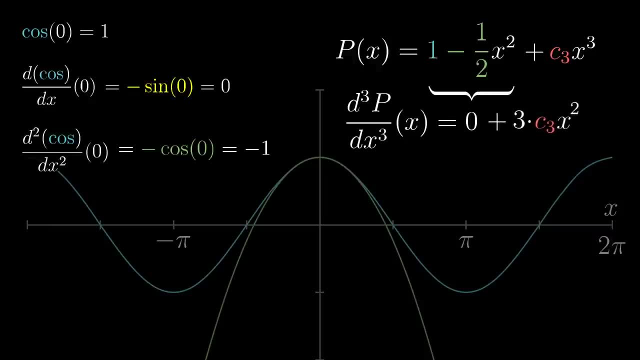 And as for that last term, after three iterations of the power rule, it looks like 1 times, 2 times, 3 times, whatever c3 is. On the other hand, the third derivative of cosine x comes out to sine of x, which equals. 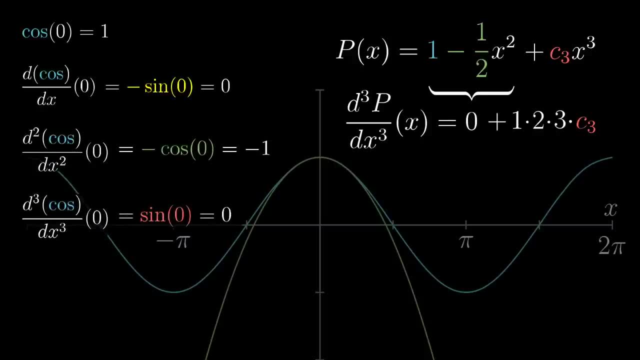 0 at x equals 0. So to make sure that the third derivatives match the constant, c3 should be 0. Or in other words, not only is 1 minus one half x squared the best possible quadratic approximation of cosine, it's also the best possible cubic approximation. 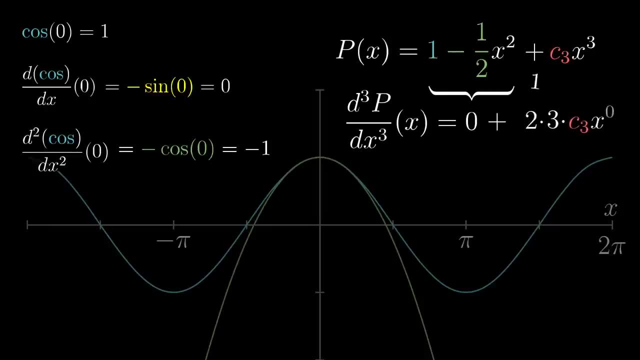 It looks like 1 times, 2 times, 3 times, whatever c3 is. On the other hand, the third derivative of cosine x comes out to sine of x, which equals 0, at x equals 0. So to make sure that the third derivatives match the constant, c3 should be 0. Or in other words, not only. 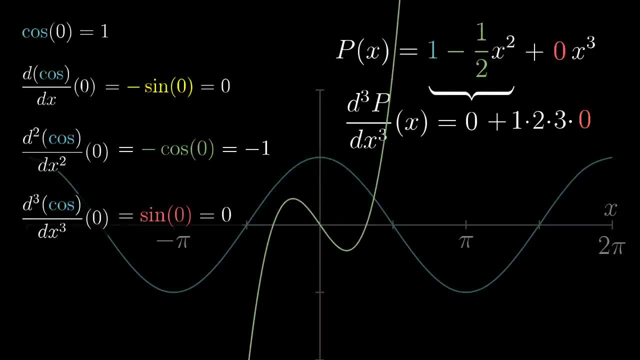 is 1 minus 1 half x squared, the best possible quadratic approximation of cosine. it's also the best possible cubic approximation. You can actually make an improvement by adding on a fourth order term- c4 times x- to the fourth. The fourth derivative of cosine is actually itself, which equals 1 at x equals. 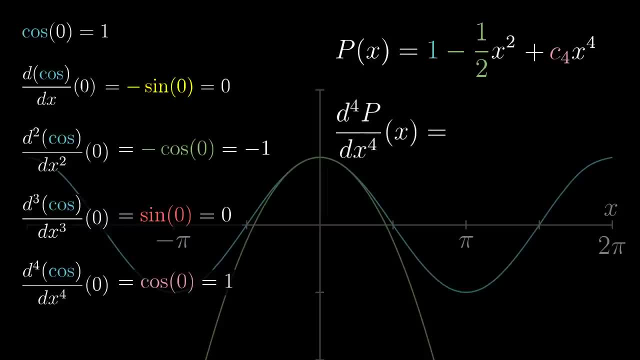 0.. And what's the fourth derivative of our polynomial with this new term? Well, when you keep applying the power rule over and over, with those exponents all hopping down in front, you end up with 1 times 2 times 3 times 4 times x squared. 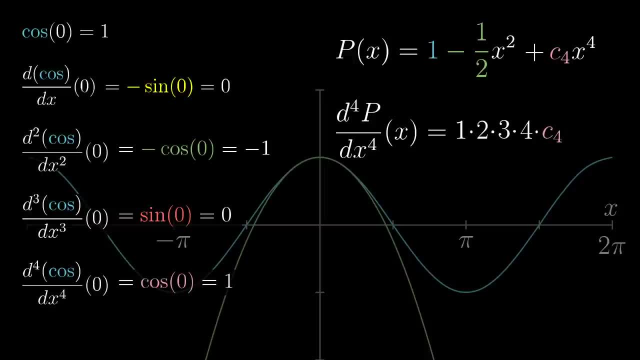 So you can actually make an improvement by adding on a fourth order term- c4 times x- to the fourth. The fourth derivative of cosine is actually itself, which equals 1, at x equals 0. So if we want this to match the fourth derivative of cosine, x, which is 1, c4 has. 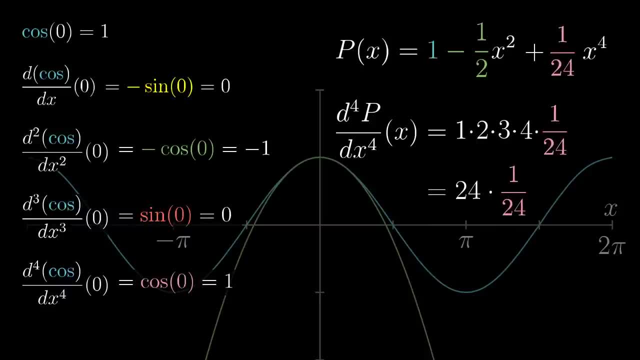 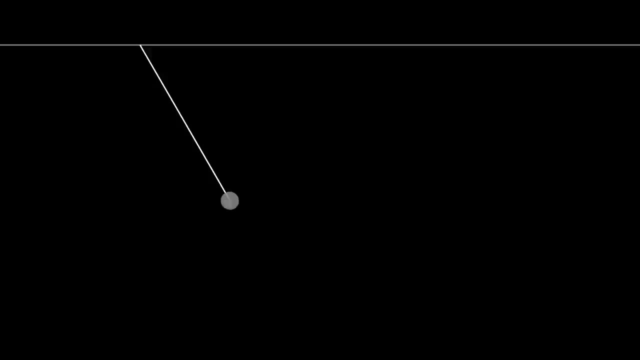 to be 1 over 24.. And indeed the polynomial 1 minus 1 half x squared plus 1 twenty-fourth times x to the fourth, which looks like this, is a very close approximation for cosine x around x equals 0.. In any physics problem involving the cosine of a small angle for 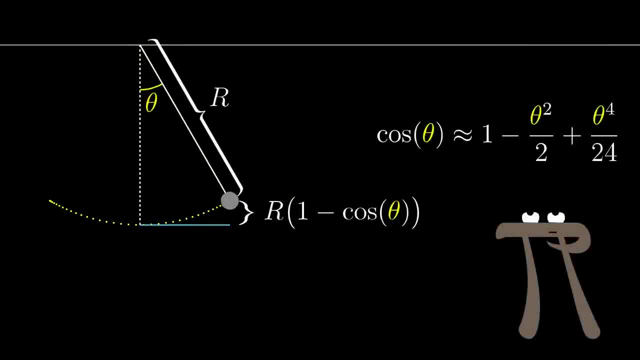 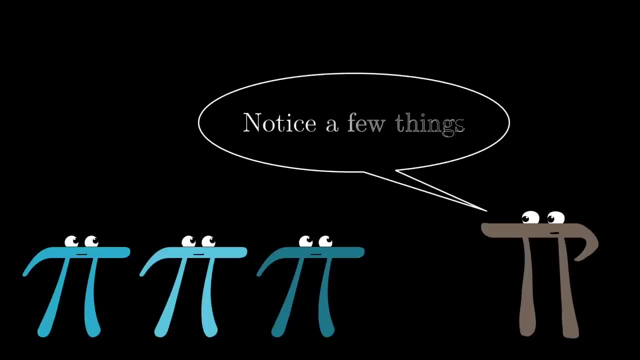 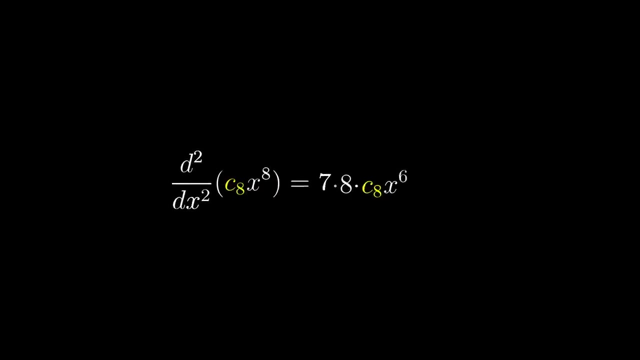 example, predictions would be almost unnoticeably different if you substituted this polynomial for cosine of x. Now take a step back and notice a few things happening with this process. First of all, factorial terms come up very naturally in this process When you take n successive derivatives. 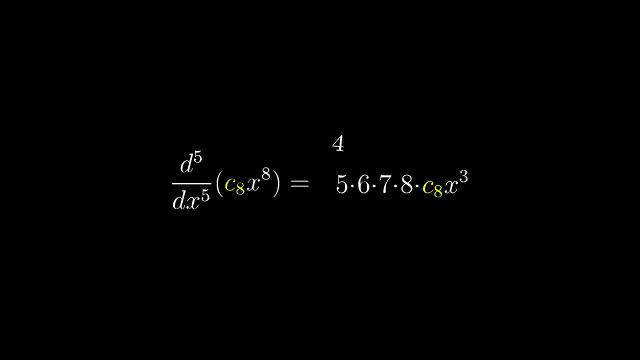 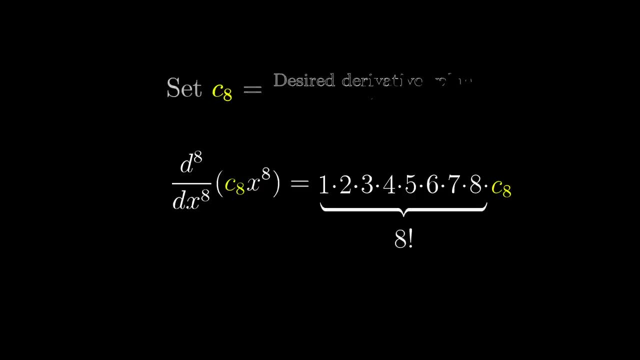 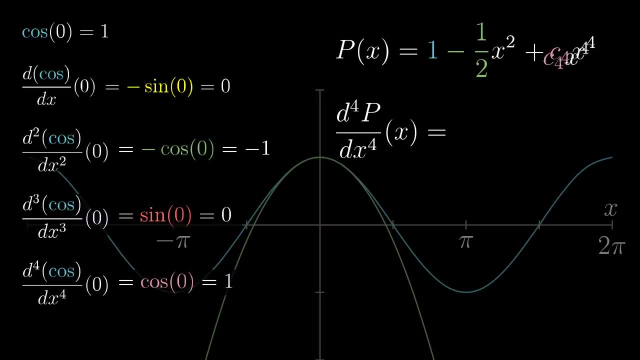 And the derivative of the polynomial is the actual derivative of the polynomial. So you don't simply set the coefficients of the polynomial equal to whatever derivative you want. You have to divide by the appropriate factorial to cancel out this effect. For example, that x to the fourth coefficient was the fourth derivative of cosine 1, but divided by 4 factorial. 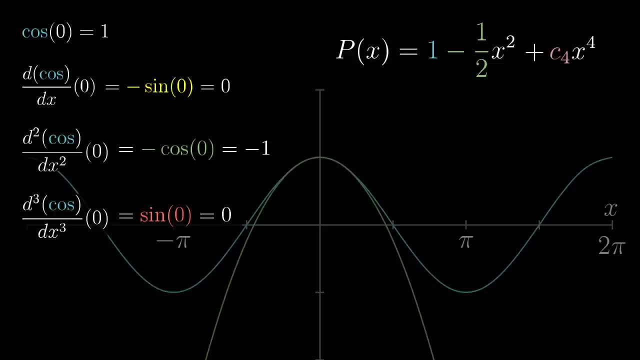 You can actually make an improvement by adding on a fourth order term, c4 times x to the fourth. The fourth derivative of cosine is actually itself, which equals 1 at x equals 0.. And what's the fourth derivative of our polynomial with this new term? 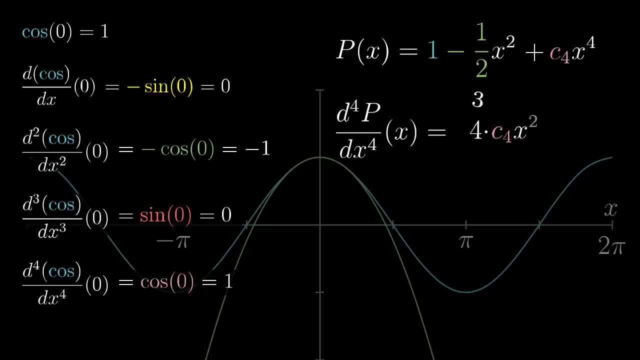 Well, when you keep applying the power rule over and over, with those exponents all hopping down in front, You end up with 1 times 2 times 3 times 4 times c4, which is 24 times c4. So if we want this to match the fourth derivative of cosine x, which is 1, c4 has to be 1 over. 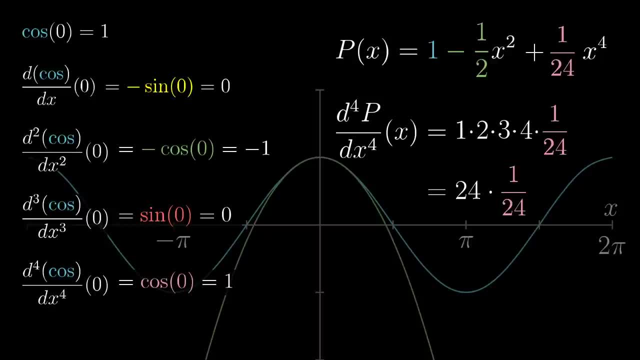 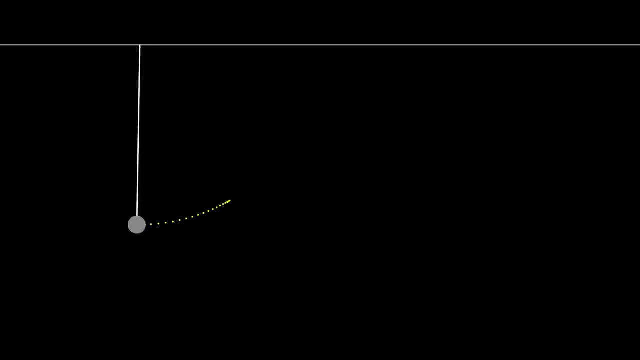 24.. And indeed the polynomial 1 minus one half x squared plus 1 twenty fourth times x to the fourth, which looks like this, is a very close approximation for cosine x around x, equals 0.. In any physics problem involving the cosine of a small angle, for example, predictions. 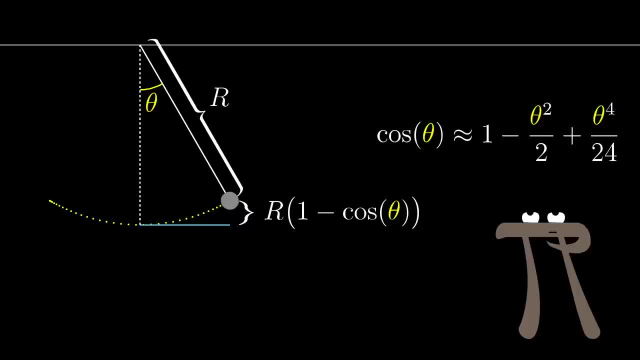 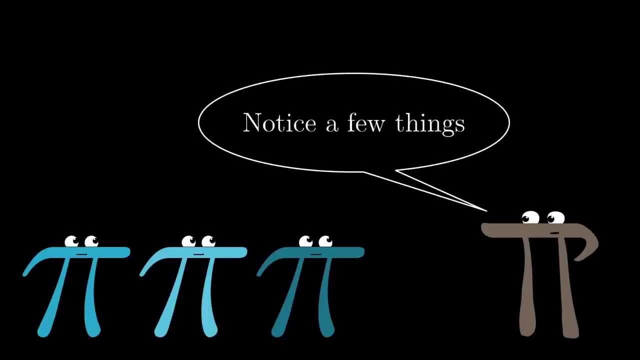 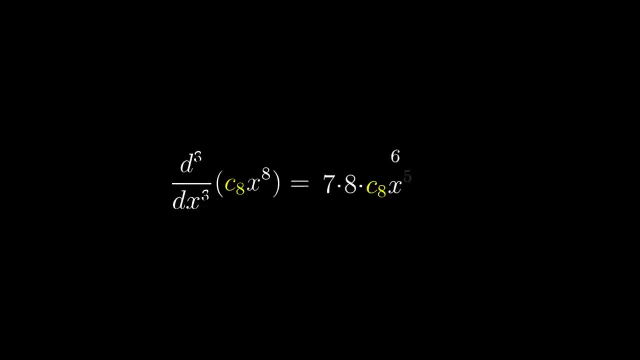 would be almost unnoticeably different if you substituted this polynomial for cosine of x. Now take a step back and notice a few things happening with this process. First of all, factorial terms come up very naturally in this process When you take n successive derivatives of the function x to the n letting the power. 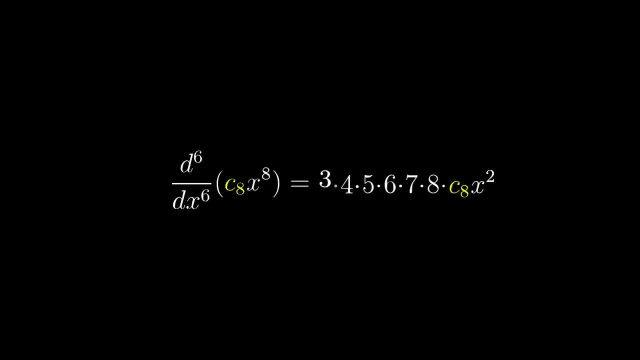 rule. just keep cascading on down. What you'll be left with is a function x to the n. What you'll be left with is a function x to the n. So that's x squared plus 1, minus x squared, which is 1 over x. 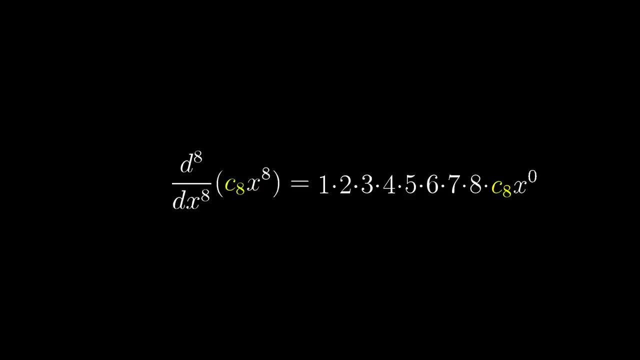 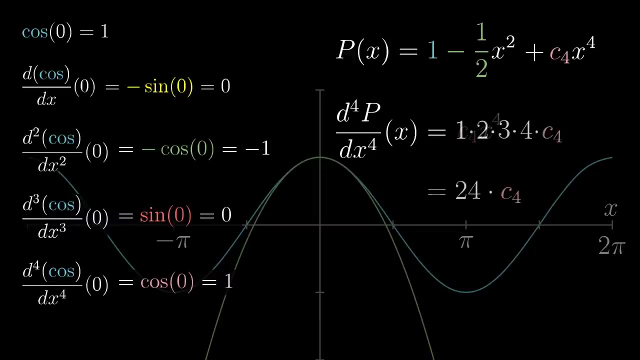 So you don't simply set the coefficients of the polynomial equal to whatever derivative you want. You have to divide by the appropriate factorial to cancel out this effect. For example, that x to the 4th coefficient was the 4th derivative of cosine 1, but divided 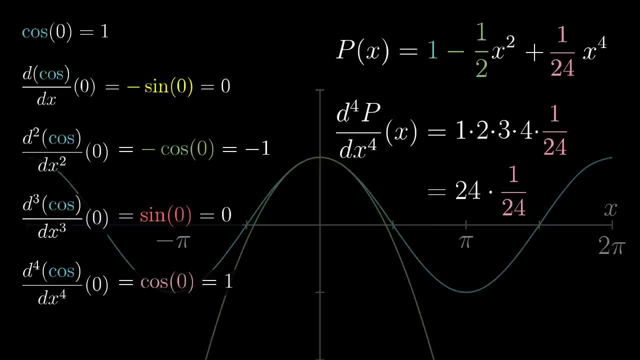 by 4, factorial 24.. But you can also consider that x to the fourth is 1 over x squared, which is also a derivative of cosine, which is 1 minus x squared by 4, so 1 divided by 4 factorial. 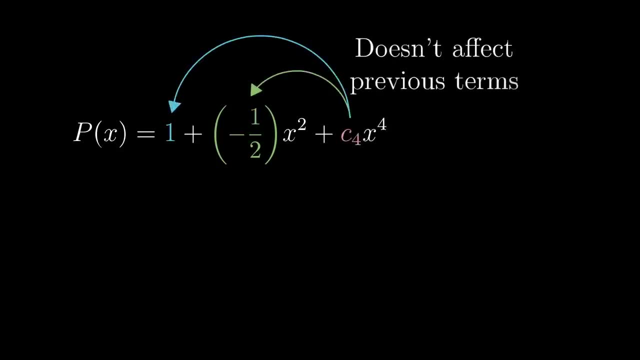 But you don't simply set the coefficients of the polynomial equal to whatever derivative, like this: c4 times x to the fourth. doesn't mess up what the old terms should be and that's really important. For example, the second derivative of this polynomial at x equals: 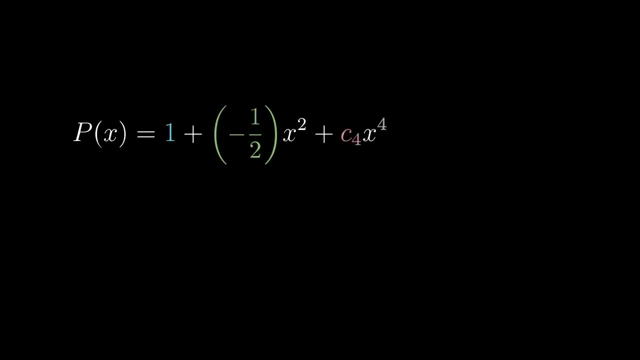 24.. The second thing to notice is that adding new terms like c4 times x to the fourth doesn't mess up what the old term means should be, And that's really important. For example, the second derivative of this polynomial, at x equals zero, is still equal to two times the second coefficient, even 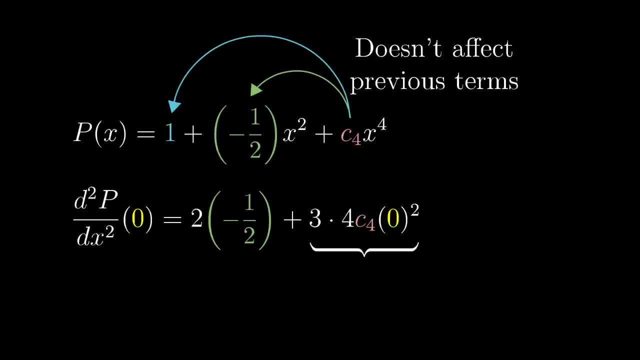 after you introduce higher order terms, And it's because we're plugging in. x equals zero, so the second derivative of any higher order term, which all include an x, will just wash away, And the same goes for any other derivative, which is why each derivative of 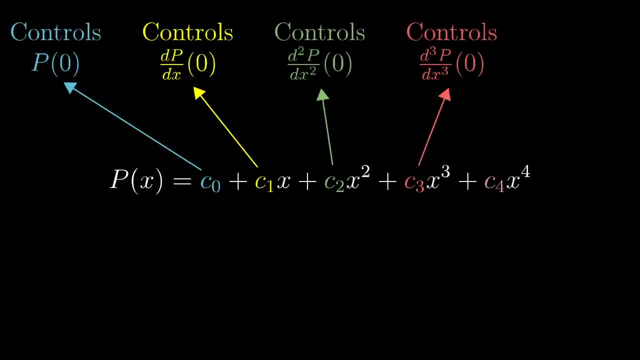 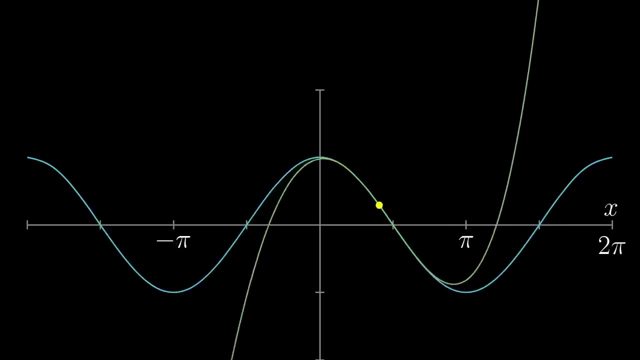 a polynomial at x equals zero is controlled by one of the coefficients. If, instead, you were approximating near an input other than zero, like maybe x equals pi, in order to get the same effect you'd have to write your polynomial in terms of. 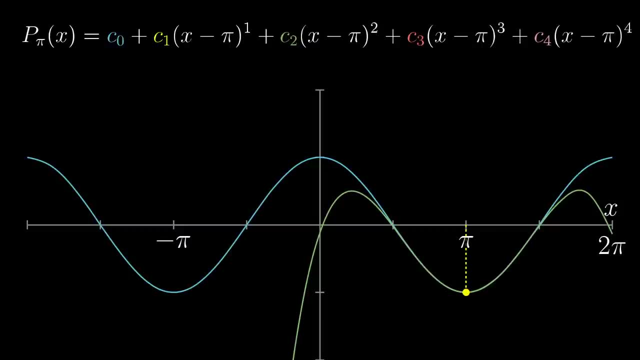 powers of x minus pi or whatever input you're looking at. This makes it look noticeably more complicated, but all we're doing is making sure that the point pi looks and behaves like zero, So that plugging in x equals pi is going to result in a lot of nice cancellation. that. 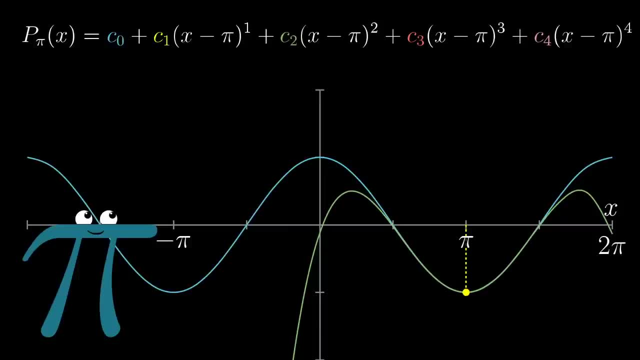 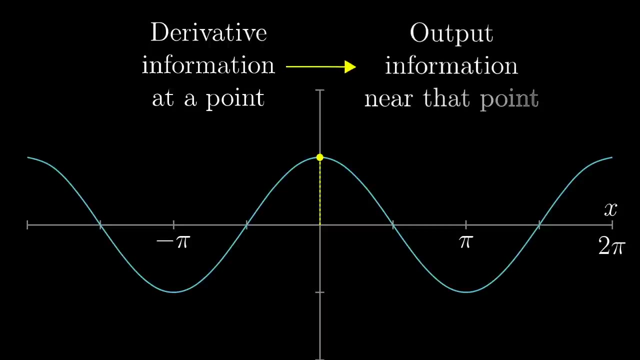 leaves only one constant. And finally, on a more philosophical level, notice how what we're doing here is basically taking information about higher order derivatives of a function at a single point and then translating that into information about the value of the function near that point. 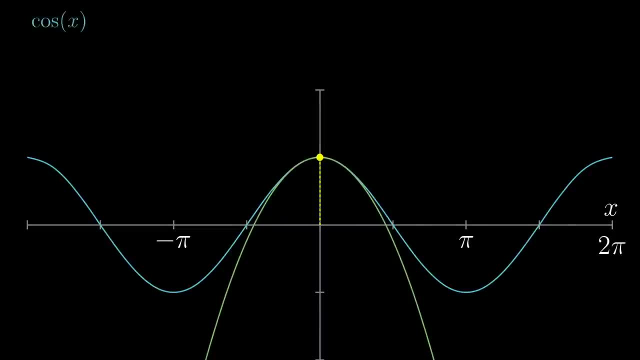 You can take as many derivatives of cosine as you want. It follows this nice cyclic pattern: Cosine of x negative sine, of x negative cosine sine, and then repeat, And the value of each one of these is easy to compute at x equals 0.. 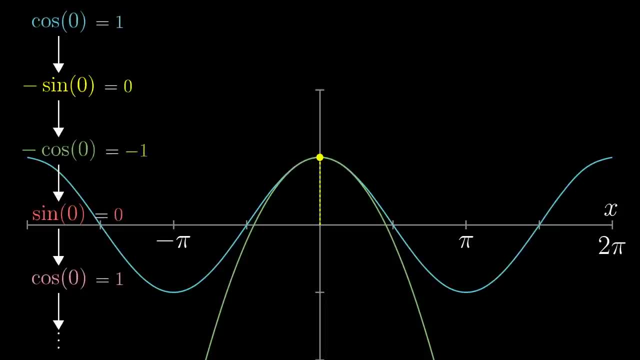 It gives this cyclic pattern 1, 0, negative 1, 0, and then repeat. And knowing the values of all of those higher order derivatives is a lot of information about cosine of x, even though it only involves plugging in a single number. 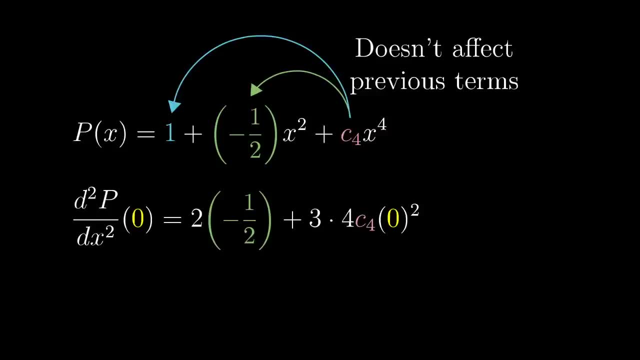 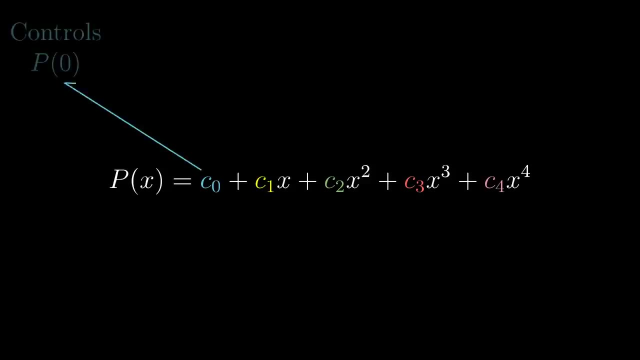 zero is still equal to two times the second coefficient, even after you introduce higher order terms, And it's because we're plugging in. x equals zero, so the second derivative of any higher order term, which all include an x, will just wash away, And the same goes for any other. 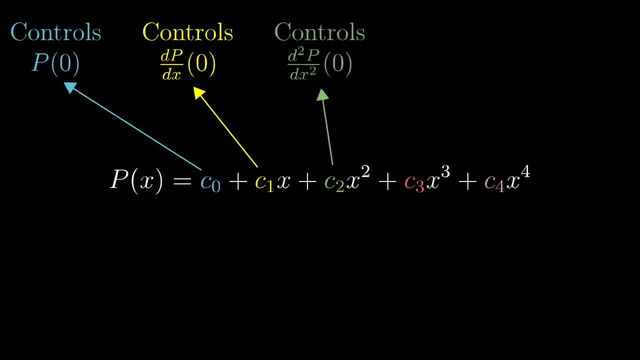 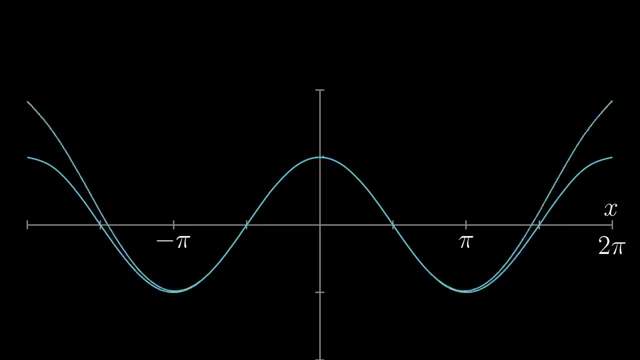 derivative, which is why each derivative of a polynomial at x equals zero is controlled by one and only one of the coefficients. If, instead, you were approximating near an input other than zero, like maybe x equals pi, in order to get the same effect you would have to write your polynomial. 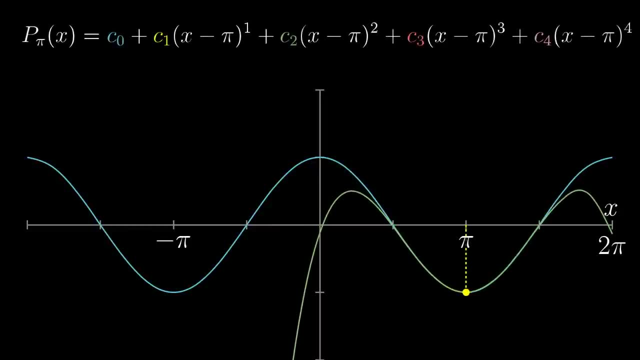 in terms of powers of x minus pi or whatever input you're looking at. This makes it look noticeably more complicated, but all we're doing is just making sure that the point pi looks and behaves like zero, so that plugging in x equals pi. 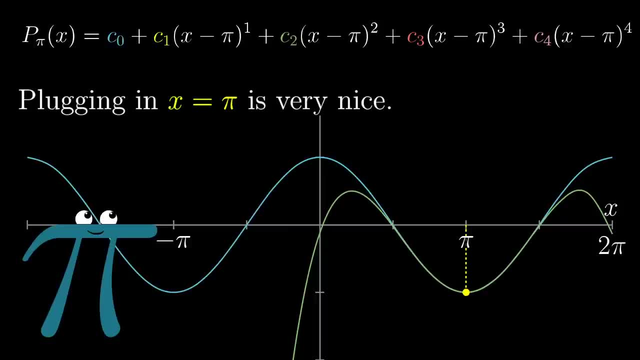 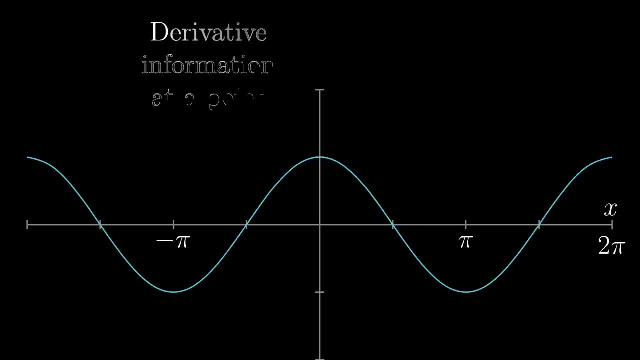 is going to result in a lot of nice cancellation that leaves only one constant. And finally, on a more philosophical level, notice how what we're doing here is basically taking information about higher order derivatives of a function at a single point and then translating that into information about the value of the function near that point. 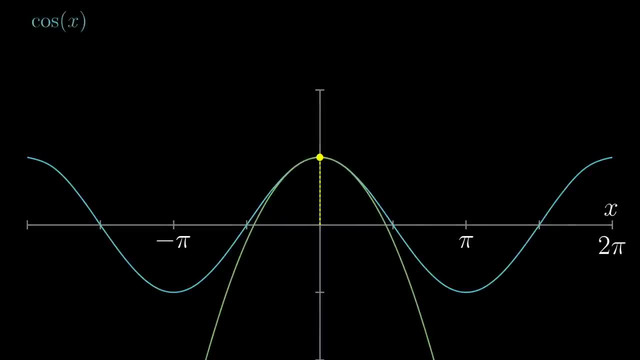 You can take as many derivatives of cosine as you want. It follows this nice cyclic pattern: cosine of x negative sine of x negative cosine sine, and then repeat, And the value of each one of these is easy to compute at. x equals zero. It gives this: 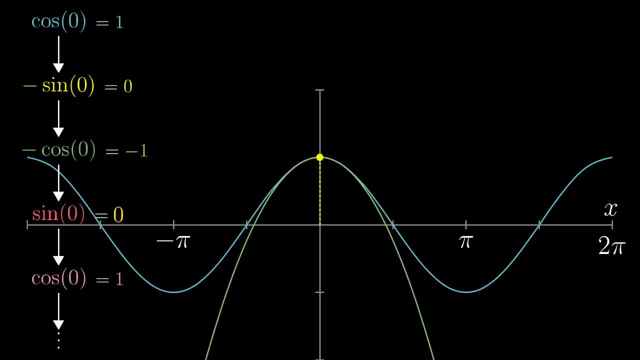 cyclic pattern: 1, 0,, negative 1, 0, and then repeat. And knowing the values of all of those higher order derivatives is a lot of information about cosine of x, even though it only involves plugging in a single number. x equals pi. 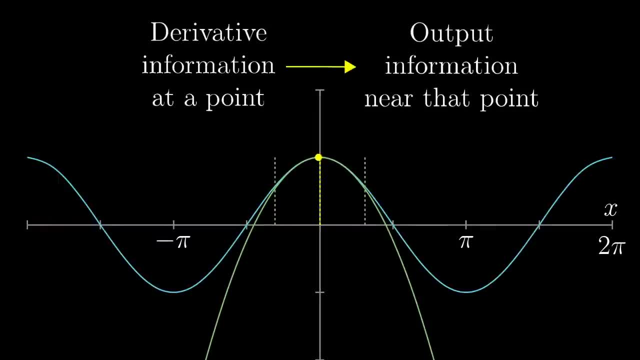 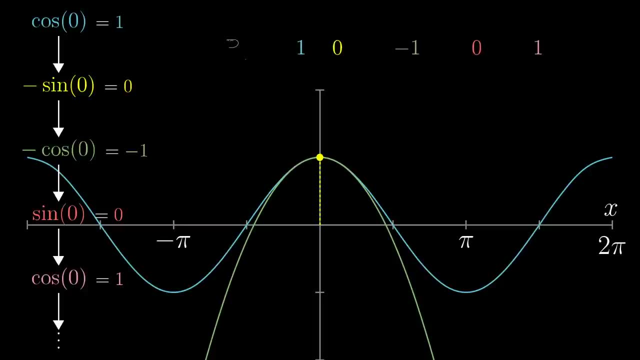 x equals zero. So what we're doing is leveraging that information to get an approximation around this input, And you do it by creating a polynomial whose higher order derivatives are designed to match up with those of cosine, following this same 1, 0, negative 1, 0 cyclic. 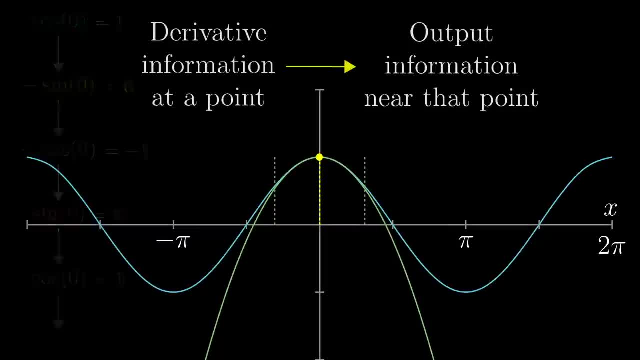 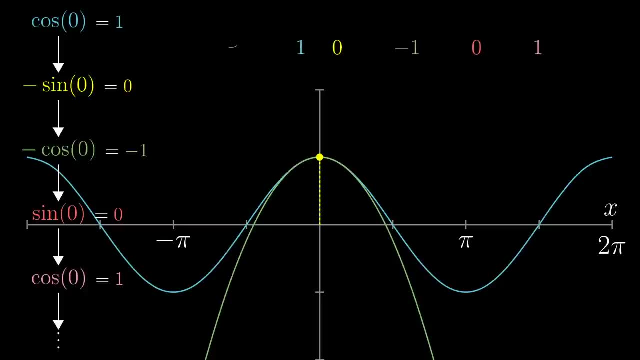 So what we're doing is leveraging that information to get an approximation around this input, And you do it by creating a polynomial whose higher order derivatives are designed to match up with those of cosine, following this same 1, 0, negative 1, 0 cyclic pattern. 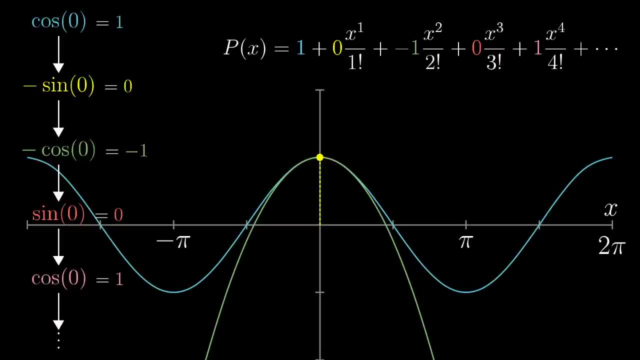 And to do that, you just make each coefficient of the polynomial follow that same pattern, but you have to divide each one by the appropriate factorial. Like I mentioned before, This is what cancels out the cascading effect of many power rule applications. 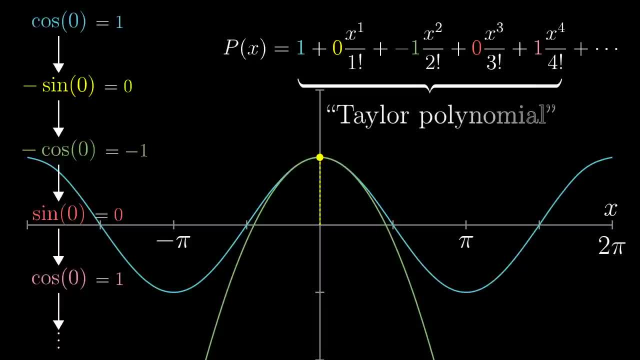 The polynomials you get by stopping this process at any point are called Taylor polynomials for cosine of x. More generally, and hence more abstractly, if we were dealing with some other function other than cosine, you would compute its derivative, its second derivative, and so on, getting 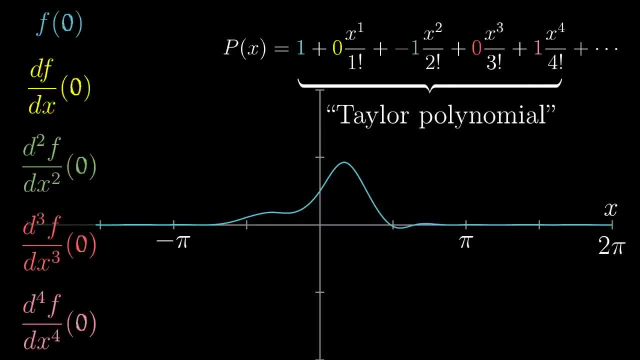 as many terms as you'd like and you would evaluate each one of them at x equals 0. Then for the polynomial approximation, you would have to do the same thing over and over For each x value or any other function being a constant term, you would have to. 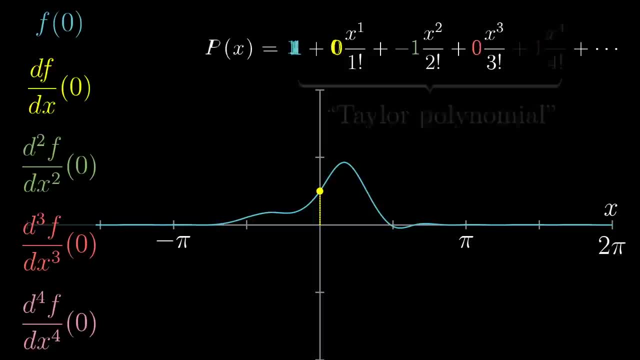 apply a función of x, so that when you multiply it you would have a function with an x that is a constant term, and then multiply this or multiply it by a function For this function, you would usually call this function the coefficient that is equal to. 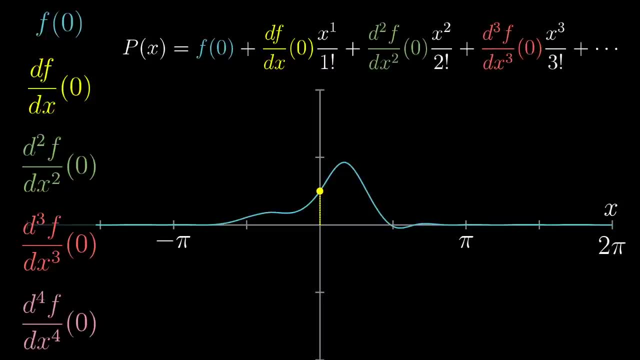 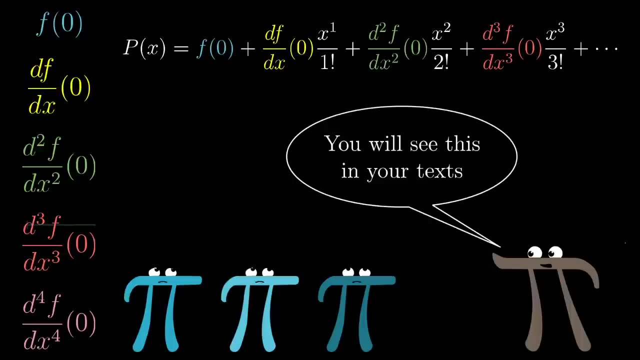 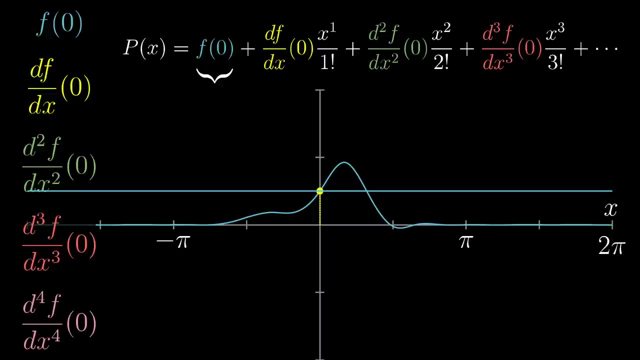 the value of the power of a function. if you want to find the power of a function In this abstract formula, you'll see the following, And when you see it, think to yourself that this constant term ensures that the value of the polynomial matches the value of f. And the second term ensures that the c-dominant function equals x. And the third term ensures that the sum of all the vaccinated terms matches the value of f. And the fourth term ensures that the sine and sine of x matches the value of the physical. 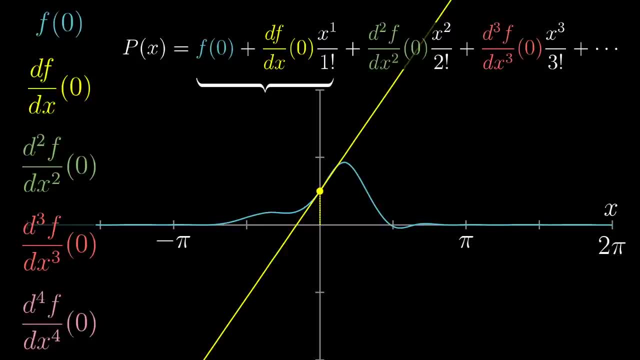 function. The slope of the polynomial matches the slope of the function. at x equals 0, the next term ensures that the rate at which the slope changes is the same at that point, and so on, depending on how many terms you want. And the more terms you choose, the closer the approximation. but the tradeoff is that 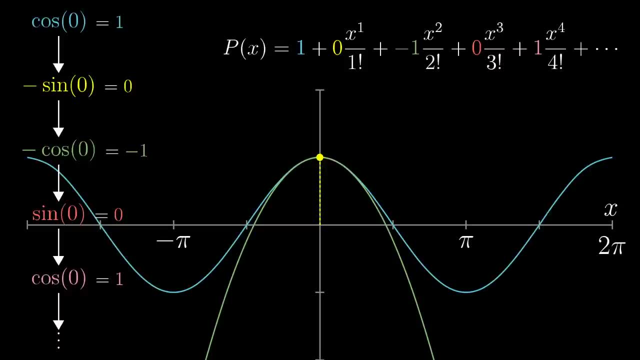 pattern, And to do that, you just make each coefficient of the polynomial follow that same pattern, but you have to divide each one by the appropriate factorial. Like I mentioned before, this is what cancels out the cascading effect of many power rule applications. 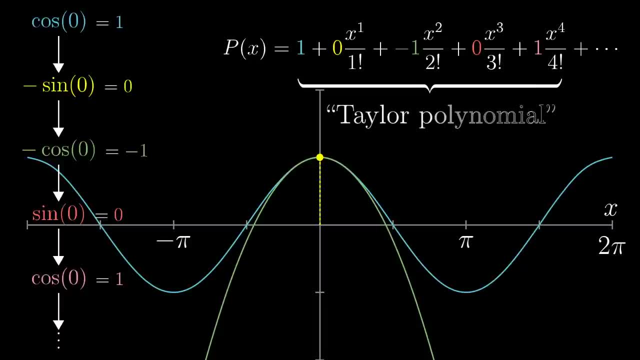 The polynomials you get by stopping this process at any point are called Taylor polynomials for cosine of x. More generally, and hence more abstractly, if we were dealing with some other function other than cosine, you would compute its derivative, its second derivative, and so on. 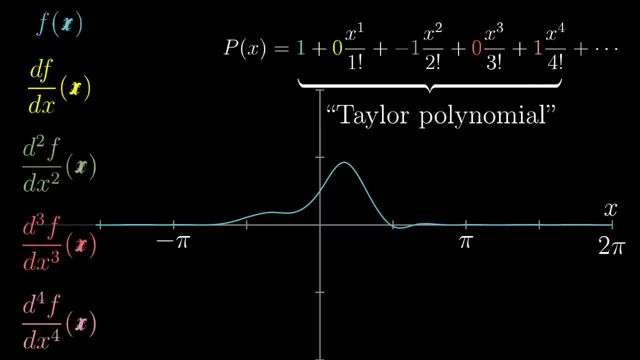 getting as many terms as you'd like and you would evaluate each one of them at x equals zero. Then, for the polynomial approximation, the coefficient of each x to the n term should be the value of the nth derivative of the function, evaluated at zero but divided by n factorial. And this whole, rather, 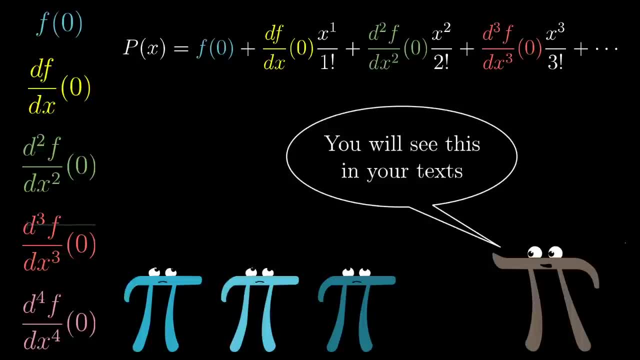 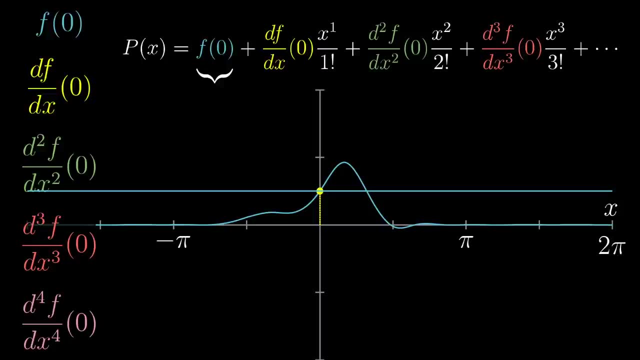 abstract formula is something that you'll likely see in any text or any course that touches on Taylor polynomials, And when you see it, I want you to think to yourself that that constant term ensures that the value of the polynomial matches with the value of f, The next term. 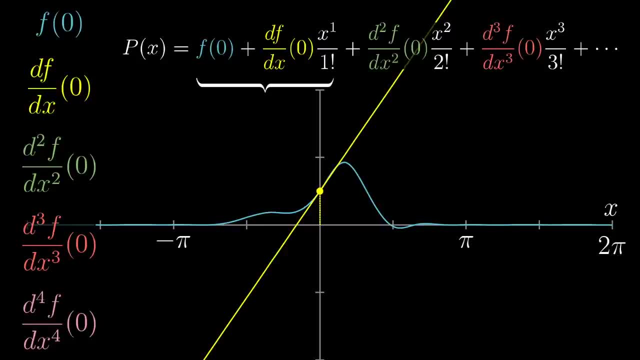 ensures that the slope of the polynomial matches the slope of the function. at x equals zero. The next term ensures that the rate at which the slope changes is the same at that point, and so on, depending on how many terms you want. And the more terms you choose, the closer the approximation. 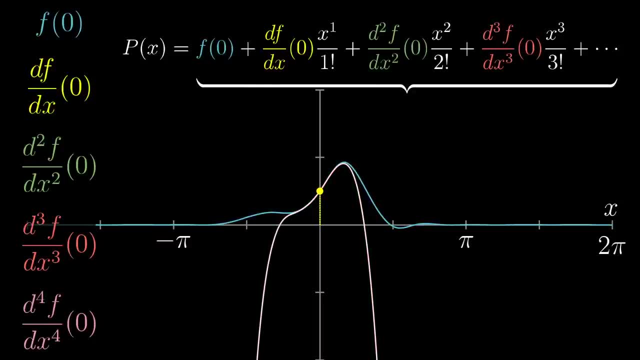 but the tradeoff is that the polynomial you'd get would be more complicated. And, to make things even more general, if you wanted to approximate near some input other than zero, which we'll call a, you would write this polynomial in terms of powers of x minus a and you would evaluate all the 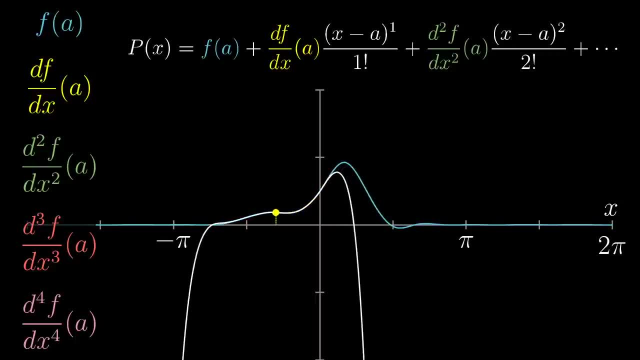 derivatives of f at that input a. This is what Taylor polynomials look like in their fullest generality: Changing the value of a. changes where this approximation is hugging the original function, where its higher-order derivatives will be equal to those of the original function. 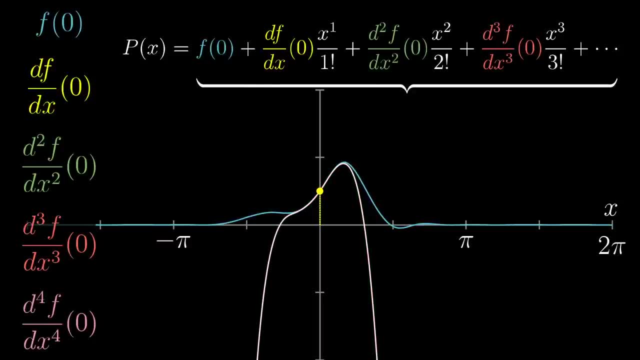 the polynomial you'd get would be more complicated And, to make things even more general, if you wanted to approximate near some input other than 0, which we'll call a, you would write this polynomial in terms of powers of x minus a and you would evaluate all the derivatives of f at that input, a. 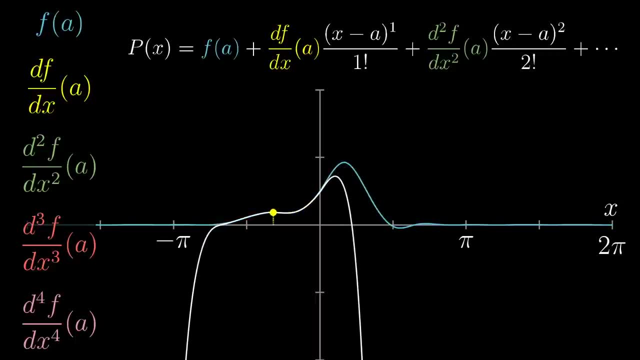 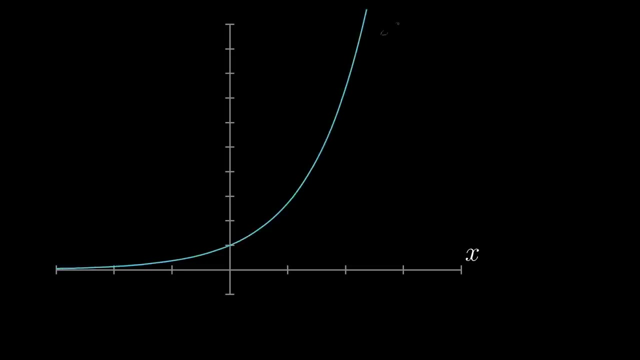 This is what Taylor polynomials look like in their fullest generality: Changing the value of a, changes where this approximation is hugging the original function, where its higher-order derivatives will be equal to those of the original function. One of the simplest meanings of Taylor polynomials can be found in this example. 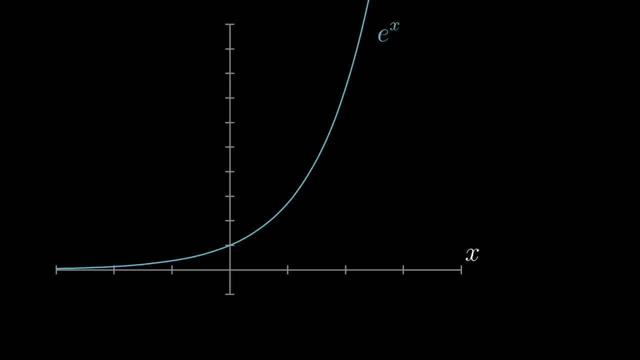 One of the most meaningful examples of this is the function e to the x. around the input, x equals 0. Computing the derivatives is super nice, as nice as it gets, because the derivative of e to the x is itself, so the second derivative is also e to the x, as is its third and so 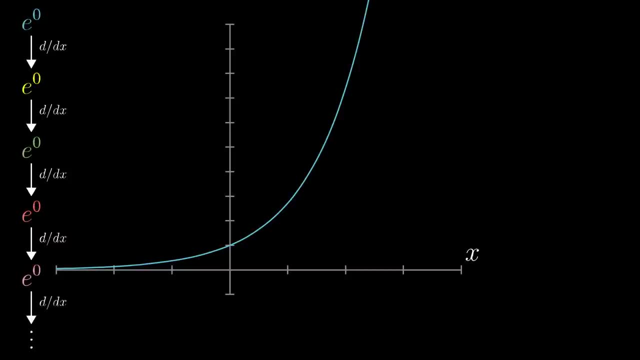 on. So at the point, x equals 0,. all of these are equal to 1.. And what that means is our polynomial approximation should look like: 1 plus 1 times x, plus 1 over 2 times x squared, plus 1 over 3 factorial times x cubed, and so on, depending on how. 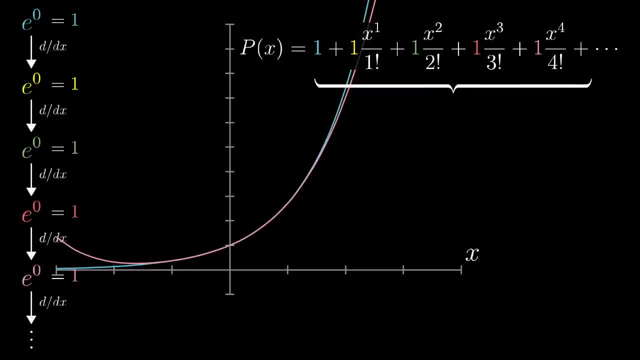 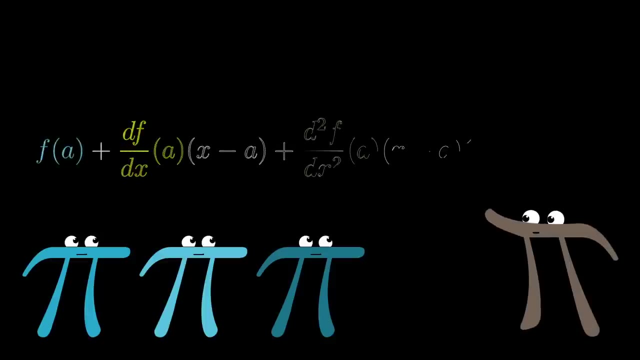 many terms you want. These are the Taylor polynomials for e to the x. Okay, so with that as a foundation, in the spirit of showing you just how connected all the topics of calculus are, let me turn to something kind of fun, a completely different. 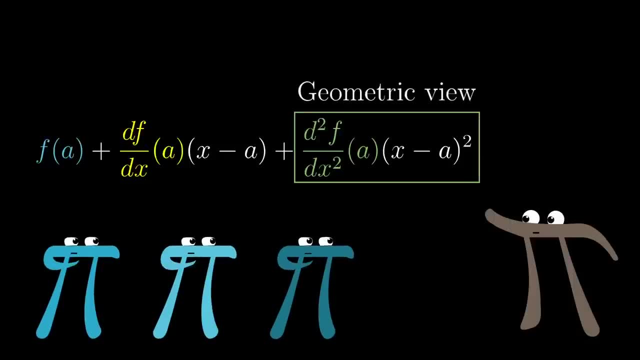 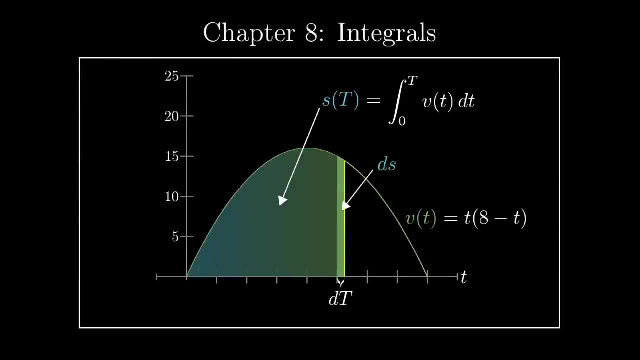 way to understand this problem. It's related to the fundamental theorem of calculus, which I talked about in chapters 1 and 8. if you need a quick refresher, Like we did in those videos, consider a function that gives the area under some graph between: 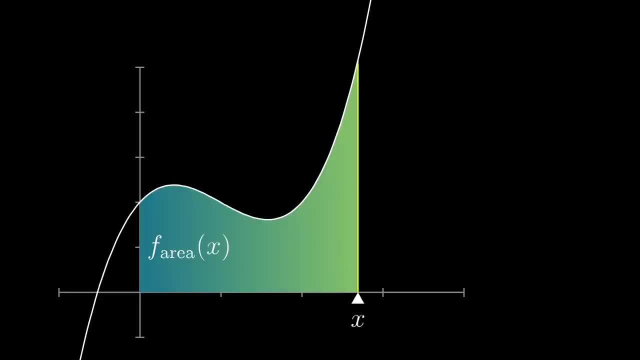 a fixed left point and a variable right point. What we're going to do here is think about how to approximate this area function, not the function for the graph itself, like we've been doing before, Focusing on that area. This is what's going to make the second-order term kind of pop-out. 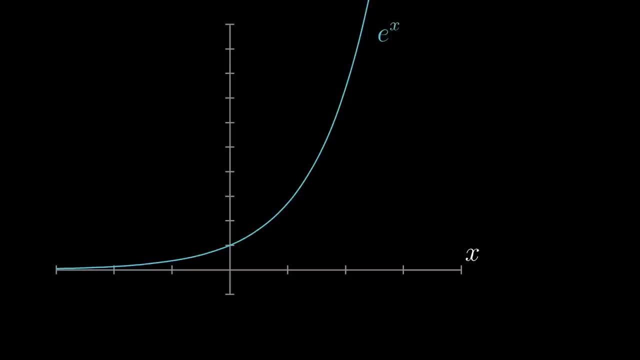 One of the simplest meaningful examples of this is the function e to the nth x around the input. x equals zero. Computing the derivatives is super nice, as nice as it gets, because the derivative of e to the x is itself. so the second derivative is also e to the x. 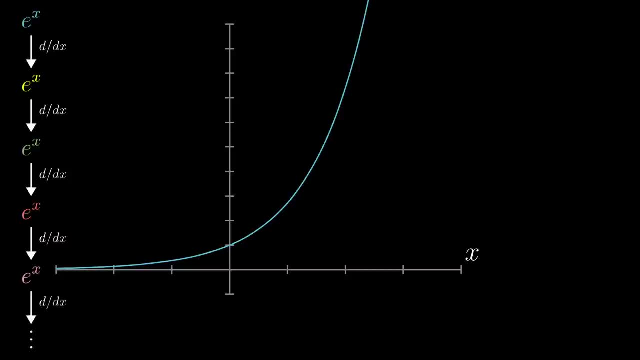 as is its third, and so on. So at the point, x equals zero. all of these are equal to one, and what that means is our polynomial approximation should look like: one plus one times x, plus one over two times x, squared plus one over three factorial times x, cubed. 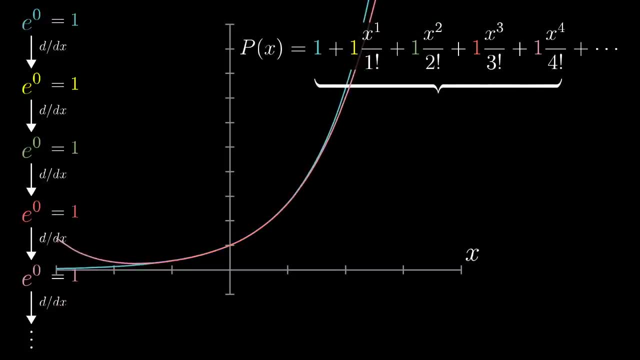 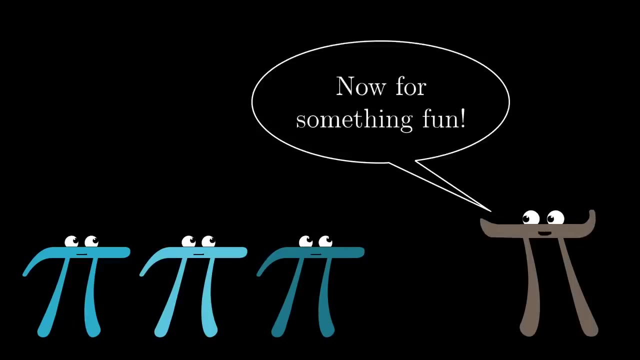 and so on, depending on how many terms you want. These are the Taylor polynomials for e to the x. Okay, so with that as a foundation, in the spirit of showing you just how connected all the topics of calculus are, let me turn to something kind of fun. 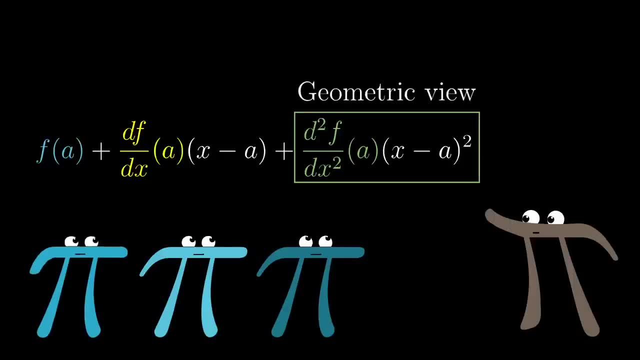 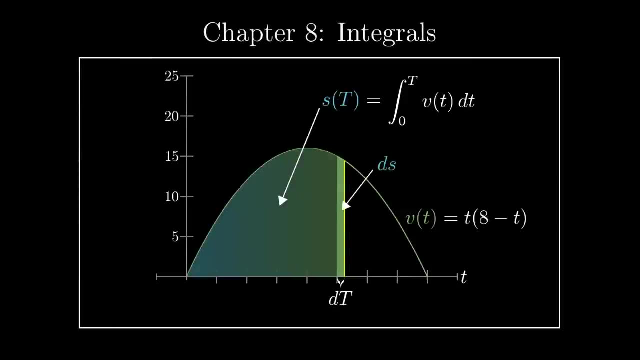 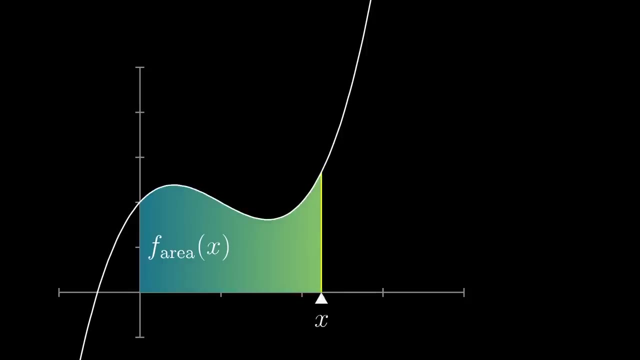 a completely different way to understand this second-order term of the Taylor polynomials, but geometrically It's related to the fundamental theorem of calculus, which I talked about in chapters 1 and 8. if you need a quick refresher, Like we did in those videos, consider a function that gives the area under some graph between a. 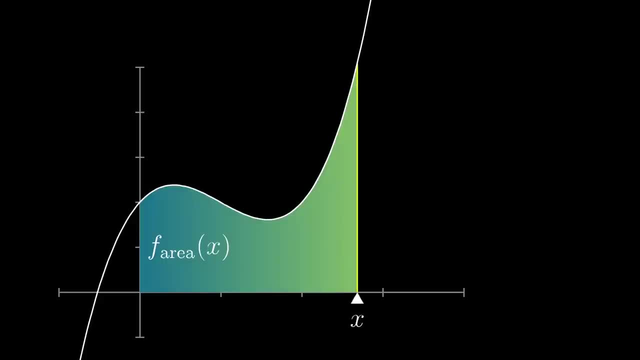 fixed left point and a variable right point. What we're going to do here is think about how to approximate this area function, not the function for the graph itself, like we've been doing before. Focusing on that area is what's going to make the second-order term kind of pop out. 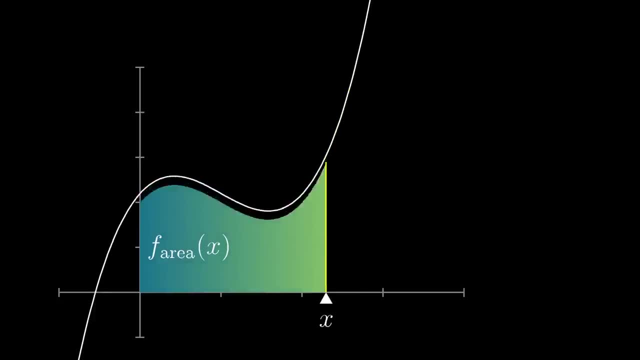 Remember, the fundamental theorem of calculus is that this graph itself represents the derivative of the area function, And it's because a slight nudge dx to the right bound of the area gives a new bit of area that's approximately equal to the height of the graph. 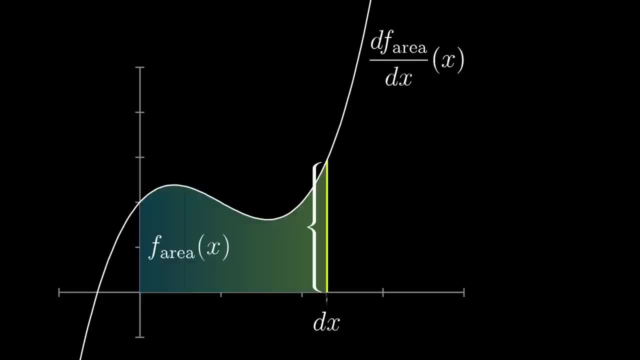 times dx And that approximation is increasingly accurate for smaller and smaller choices of dx. But if you wanted to be more accurate about this change in area, given some change in x that isn't meant to approach zero, you would have to take into account. 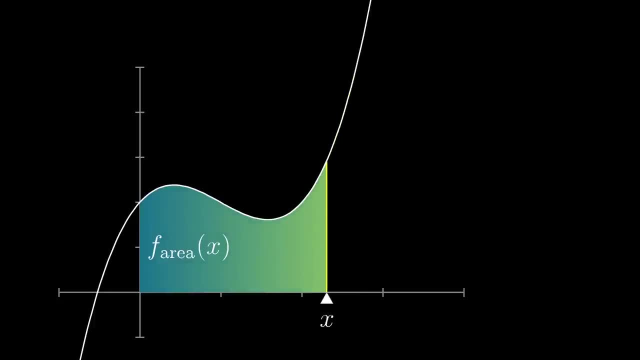 Remember, the fundamental theorem of calculus is that this graph itself represents the derivative of the area function, And it's because a slight nudge dx to the right bound of the area gives a new bit of area that's approximately equal to dx, And that approximation is increasingly accurate for smaller and smaller choices of dx. 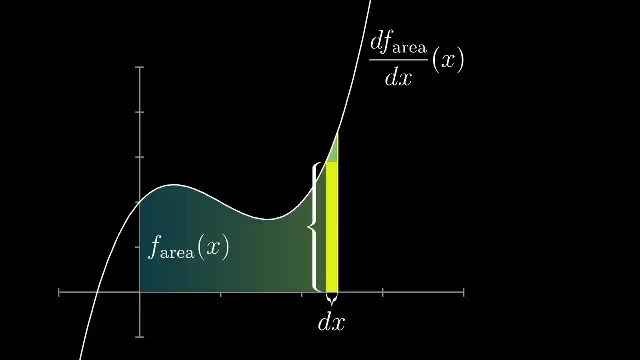 Simplified. If you wanted to be more accurate about this change in area, given some change in x that isn't meant to approach 0, you would have to take into account this portion right here, which is approximately a triangle. Let's name the starting input a and the nudged input above it, x, so that that change. 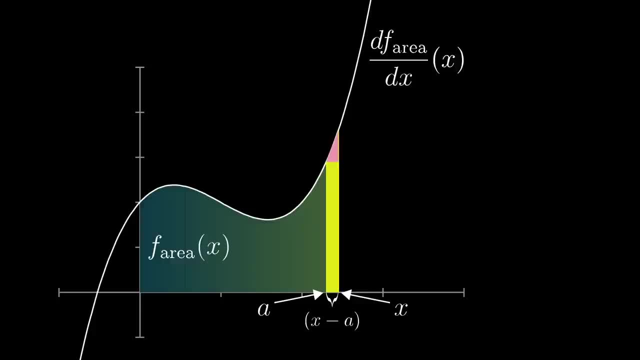 is x-a. The base of that little triangle is that change x-a and its height is the slope of the graph times x-a. Since this graph is the derivative of the area function, its slope is the second derivative of the area function evaluated at the input a. 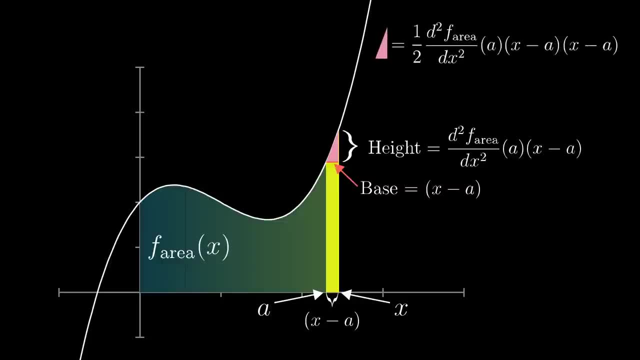 So the area of this triangle, 1 half base times height, is 1 half times the second derivative of this area function evaluated at a multiplied by x-a squared. And this is exactly what you would see with a Taylor polynomial If you knew the. 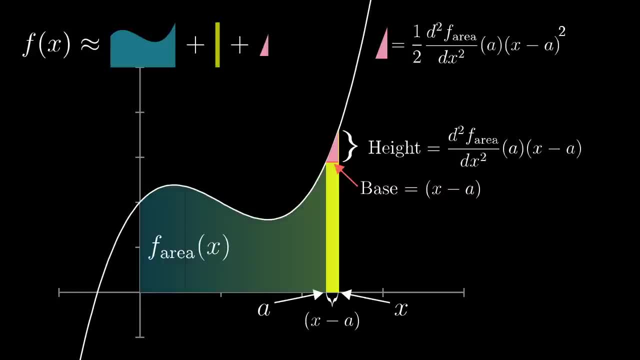 various derivative information about this area function at the point a. how would you approximate the area at the point x? Well, you have to include all that area up to a f of a, plus the area of this rectangle here, which is the first derivative times x-a, plus the area of that little triangle. 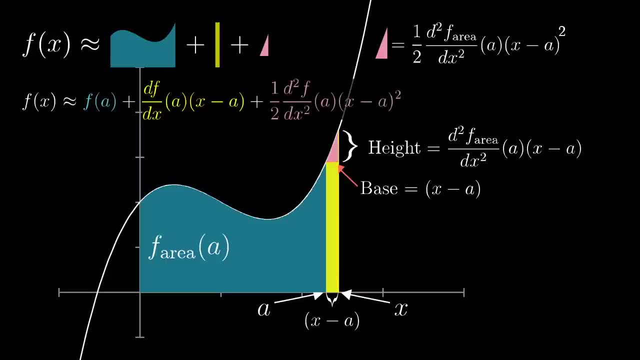 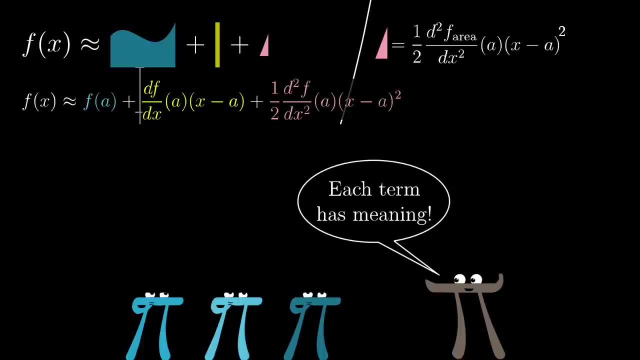 which is 1 half times the second derivative, times x-a squared. I really like this because, even though it looks a bit messy, I don't think it's a big deal. Each one of the terms has a very clear meaning that you can just point to on the diagram. 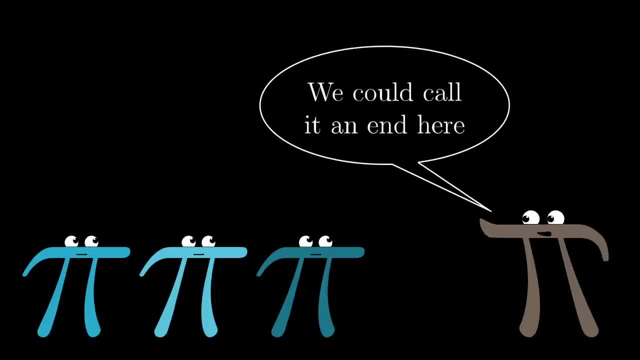 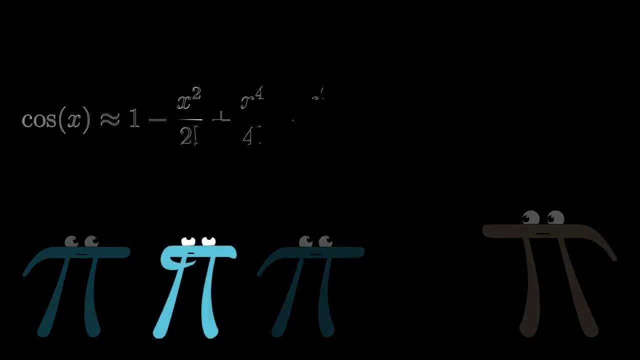 If you wanted, we could call it an end here and you would have a phenomenally useful tool for approximations with these Taylor polynomials. But if you're thinking like a mathematician, one question you might ask is whether or not it makes sense to never stop and just add infinitely many terms. 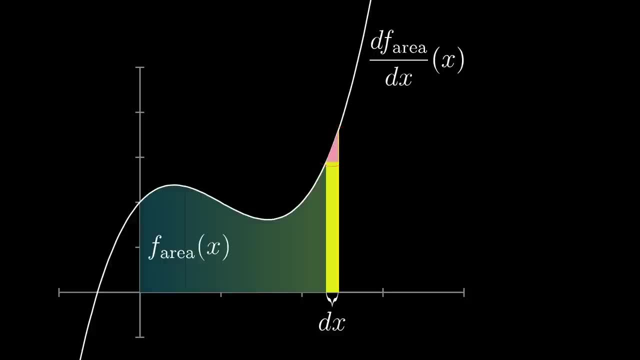 this portion right here which is approximately a triangle. Let's name the starting input, a, and the nudged input above it, x, so that that change is x-a. The base of that little triangle is that change x-a, and its height is the slope of the graph. times x-a. Since this graph is a triangle, it's not a triangle, but it's a triangle. Since this graph is a triangle, it's a triangle and its height is the slope of the graph. times x-a, Since this graph. 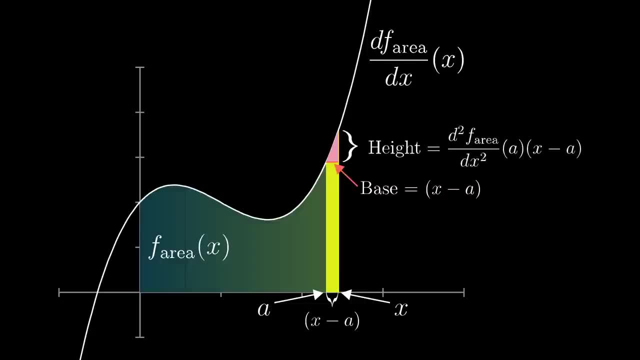 is the derivative of the area function. its slope is the second derivative of the area function evaluated at the input a. So the area of this triangle- 1 half base times height, is 1 half times the second derivative of this area function evaluated at a multiplied by x-a squared. 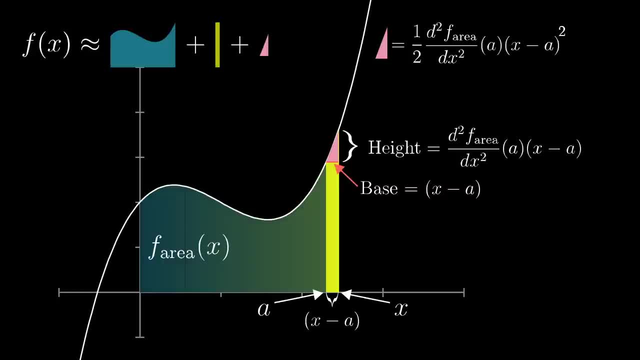 And this is exactly what you would see with a Taylor polynomial. If you knew the various derivative information about this area function at the point a, how would you approximate the area at the point x? Well, you have to include all that area up to a f of a, plus the area of this rectangle here. 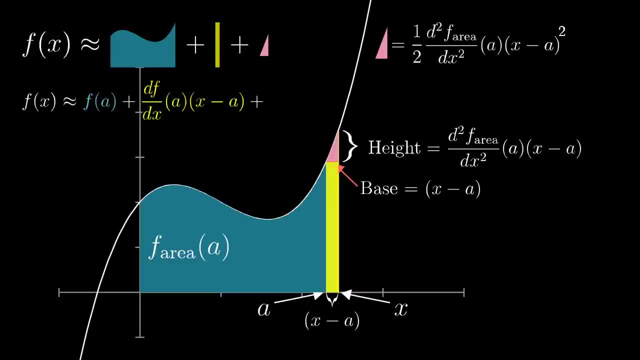 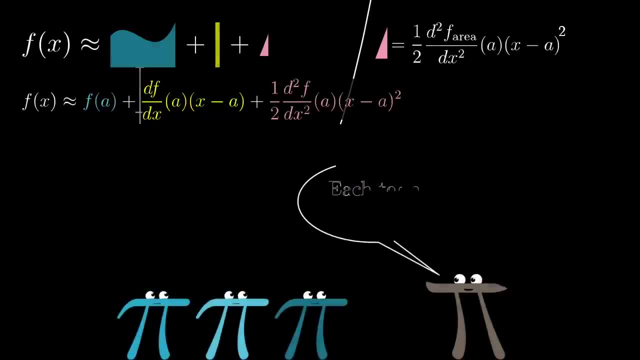 which is the first derivative times x-a, plus the area of that little triangle which is 1 half times the second derivative times x-a squared. I really like this because, even though it looks a bit messy all written out, each one of the terms has a very clear meaning: that 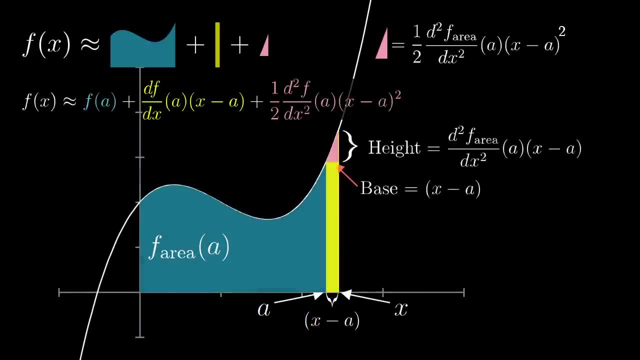 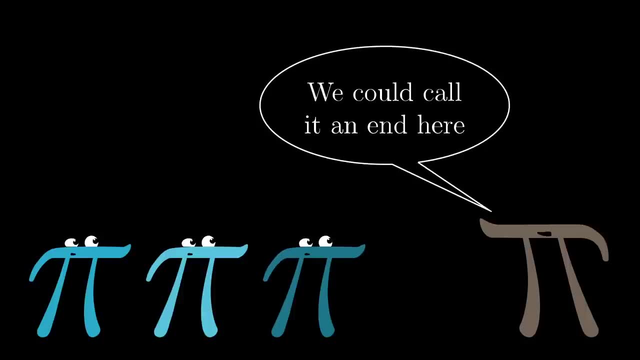 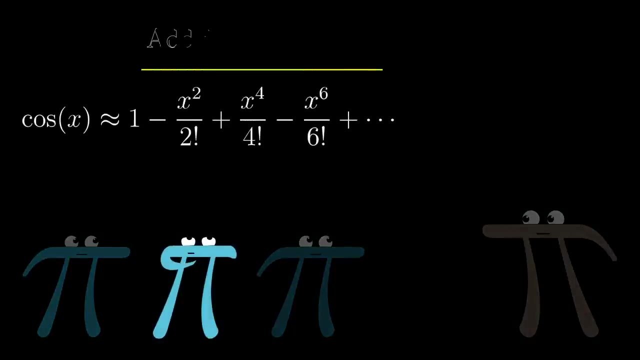 you can just point to on the diagram. If you wanted, we could call it an end here and you would have a phenomenally useful tool for approximations with these Taylor polynomials. But if you're thinking like a mathematician, one question you might ask is whether or not it makes sense to never stop. 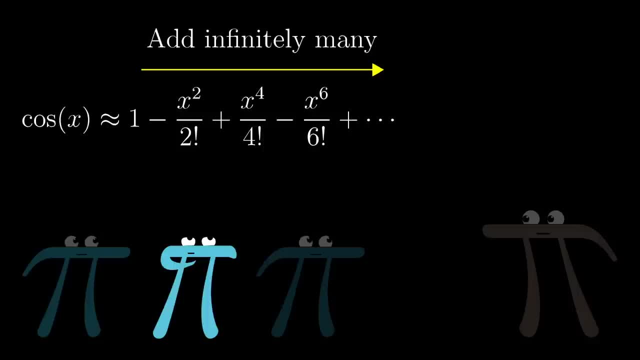 and just add infinitely many terms. In math, an infinite sum is called a series. so even though one of these approximations with finitely many terms is called a Taylor, adding all infinitely many terms gives what's called a Taylor series. You have to be really careful with the idea of an infinite series, because it doesn't actually make. 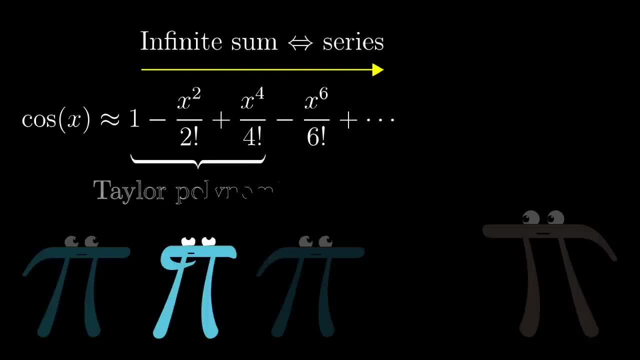 In math, an infinite sum is called a series. So what is a series? Well, even though one of these approximations with finitely many terms is called a Taylor polynomial, adding all infinitely many terms gives what's called a Taylor series. 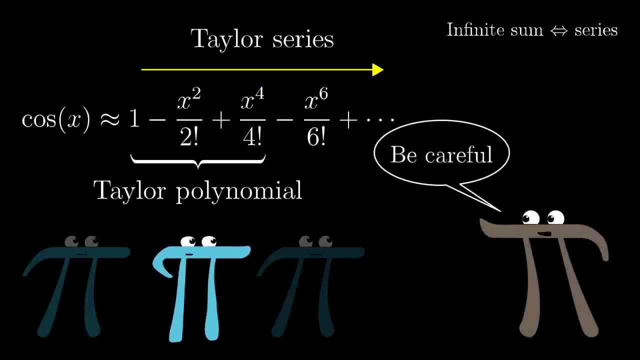 You have to be really careful with the idea of an infinite series, because it doesn't actually make sense to add infinitely many things. You can only hit the plus button on the calculator so many times, But if you have a series where adding more and more of the terms which makes sense at 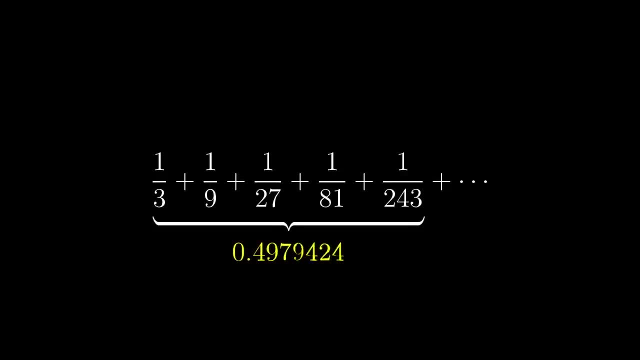 each step gets you increasingly close to some specific reason. So if you have a series where adding more and more of the terms which makes sense at each step gets you increasingly close to some specific reason. So if you have a series where adding more and more of the terms which makes sense, 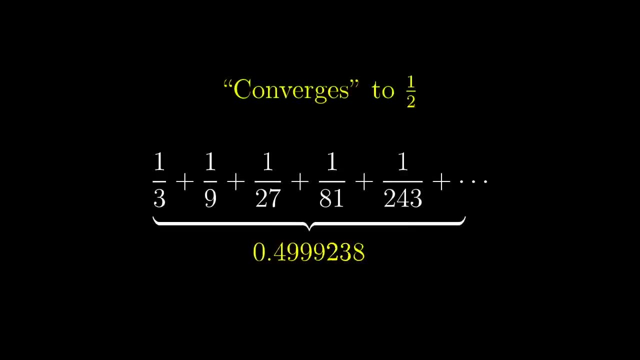 at each step gets you increasingly close to some specific reason. So if you have a series where adding more and more of the terms which makes sense at each step gets you increasingly close to some specific reason, Or if you're comfortable extending the definition of equality to include this kind of series. 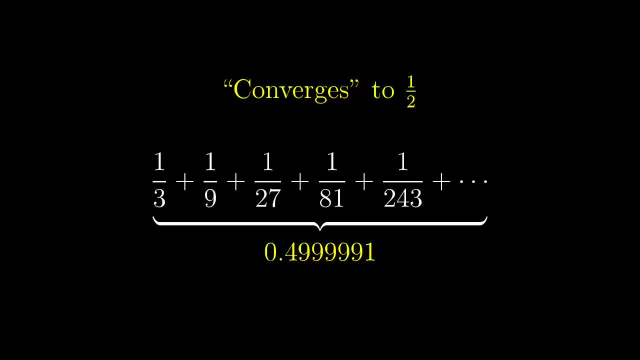 convergence, you'd say that the series as a whole, the infinite sum, equals the values that it's converging to. For example, look at the Taylor polynomial for e to the x and plug in some input like: x equals 1.. As you add more and more polynomial terms, the total sum becomes more and more infinite, and you can add more and more of the terms and the number of others that you add. So the total sum is eventually equal to e, to the x. 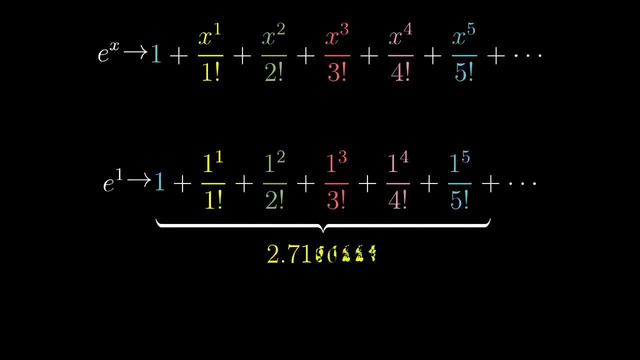 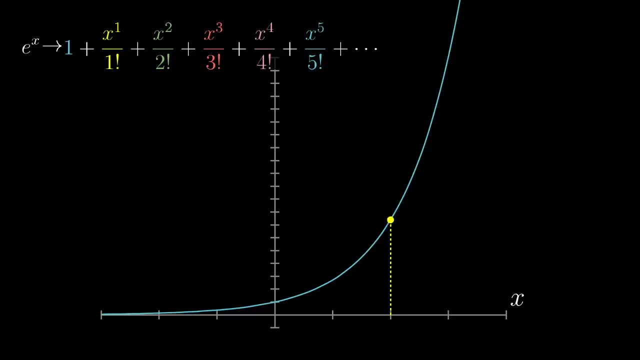 But consider other terms as well. total sum gets closer and closer to the value e. so you say that this infinite series converges to the number e, or what's saying the same thing, that it equals the number e. In fact, it turns out that if you plug in any other value of x, like x equals 2, and 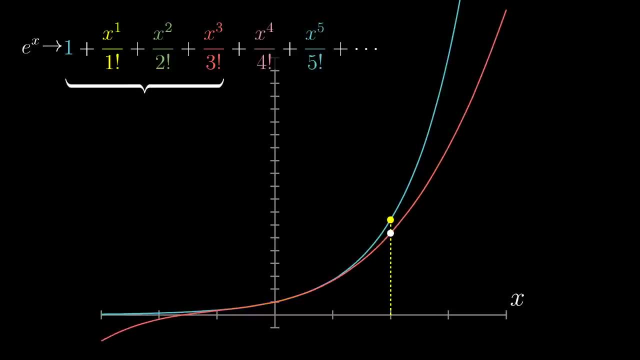 look at the value of the higher and higher order Taylor polynomials. at this value, they will converge towards e, to the x, which in this case is e squared, And this is true for any input, no matter how far away from zero it is, even though 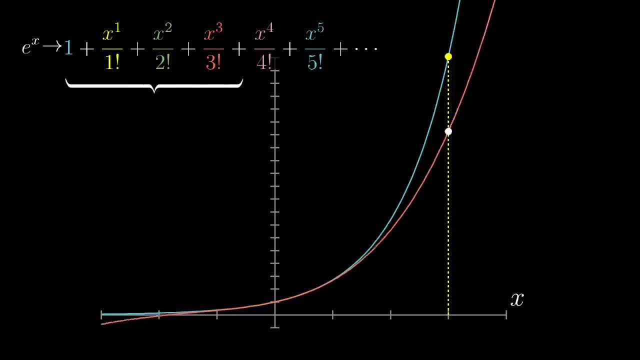 these Taylor polynomials are constructed only from derivative information gathered at the input zero. In a case like this, we say that e to the x equals its own Taylor series at all inputs x, which is kind of a magical thing to have happen. And even though 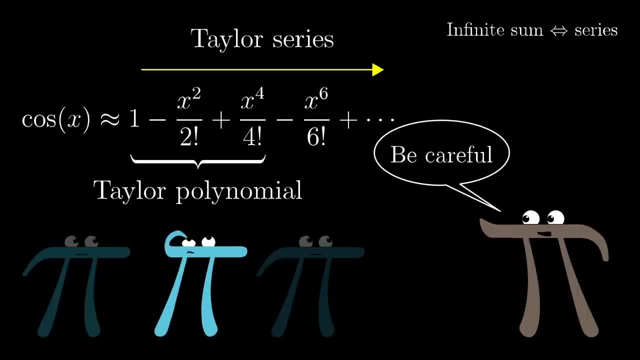 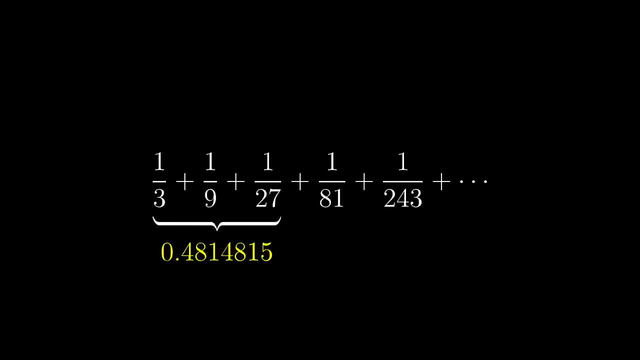 sense to add infinitely many things. You can only hit the plus button on the calculator so many times. But if you have a series where adding more and more of the terms which makes sense at each step gets you increasingly close to some specific value, what you say is that the series converges to. 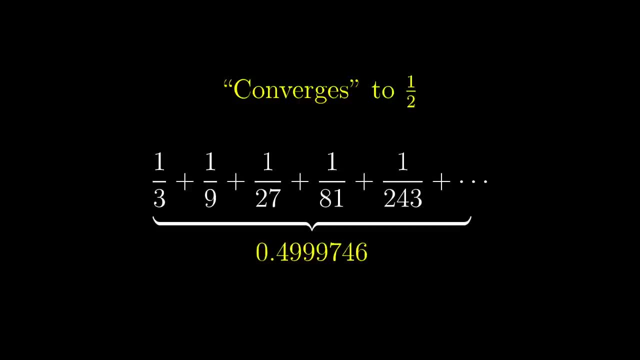 that value. Or if you're comfortable with extending the definition of equality to include this kind of series convergence, you'd say that the series as a whole, this infinite sum, equals the value that it's converging to. For example, look at the Taylor polynomial for e. 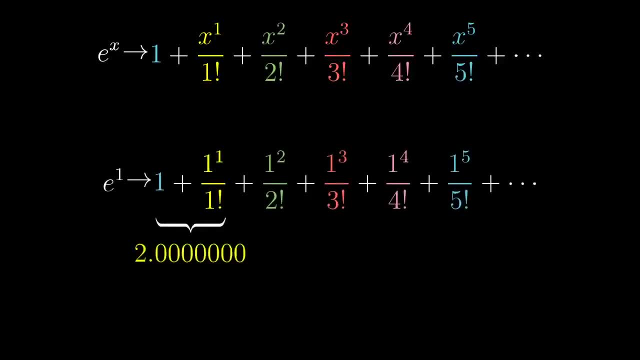 to the x and plug in some input like: x equals 1.. As you add more and more polynomial terms, the total sum gets closer and closer to the value e. that this infinite series converges to the number e, or what's saying the same thing? 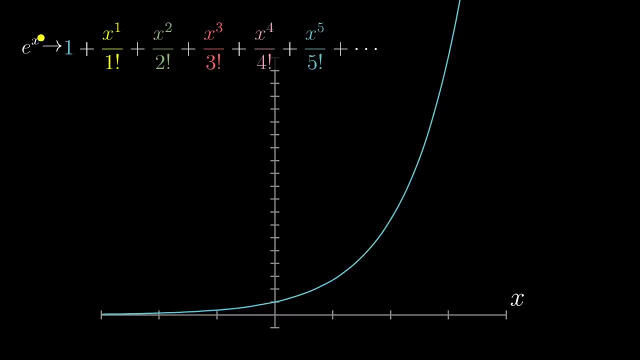 that it equals the number e. In fact, it turns out that if you plug in any other value of x, like x equals 2, and look at the value of the higher and higher order Taylor polynomials, at this value they will converge towards e, to the x, which in this case is e squared. 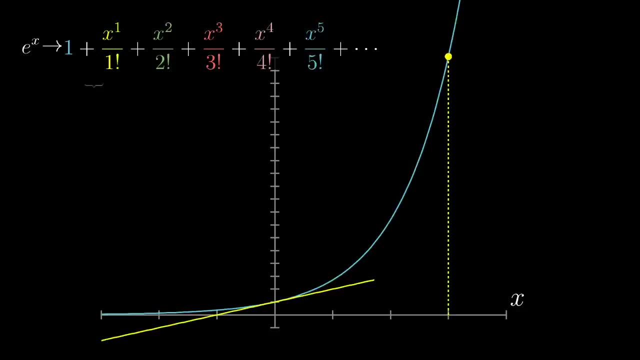 And this is true for any input, no matter how far away from 0 it is, even though these Taylor polynomials are constructed only from derivative information gathered at the input 0. In a case like this, we say that e to the x equals its own Taylor series at all inputs. 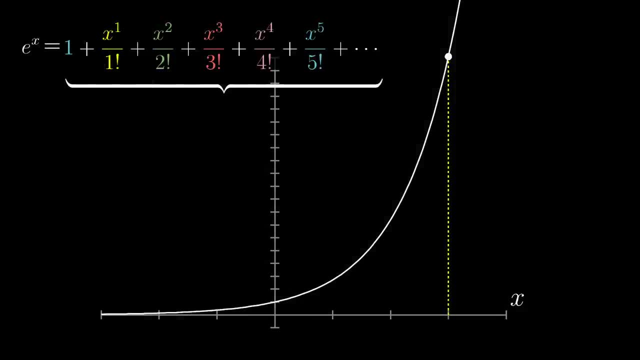 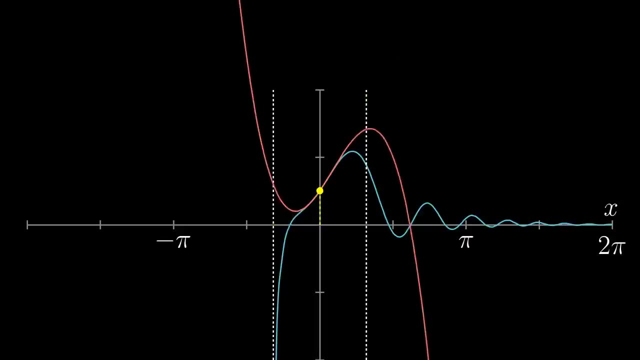 x, which is kind of a magical thing to have happen, And even though this is also true for a couple other important functions, things like sine and cosine. sometimes these series only converge within a certain range around the input whose derivative information you're using. If you work out the Taylor series for the natural log of x around the input, x equals. 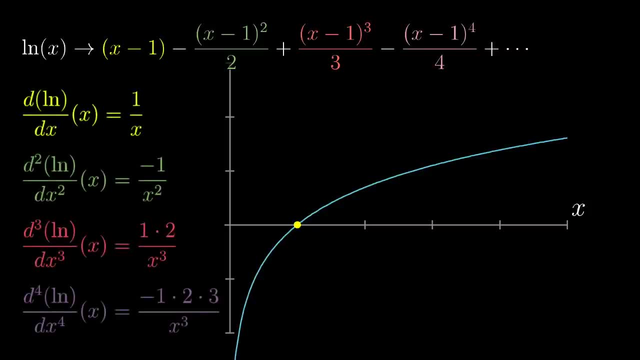 1,, which is built by evaluating the higher order derivatives of the natural log of x at x equals 1,. this is what it would look like When you plug in an input between 0 and 2,. adding more and more terms of this series will indeed get you closer and closer. 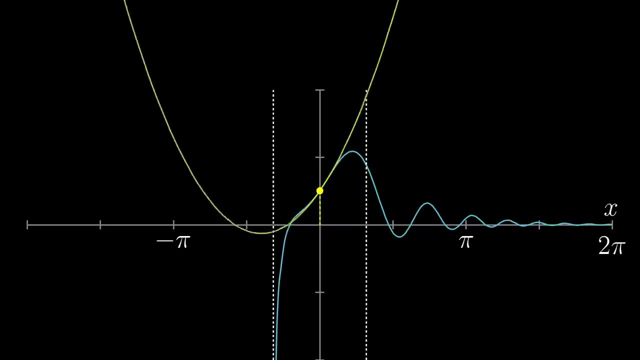 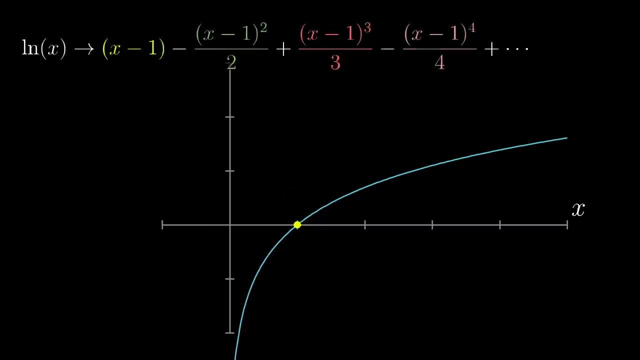 this is also true for a couple other important functions, things like sine and cosine. sometimes these series only converge within a certain range around the input whose derivative information you're using. If you work out the Taylor series for the natural log of x around the input, x equals. 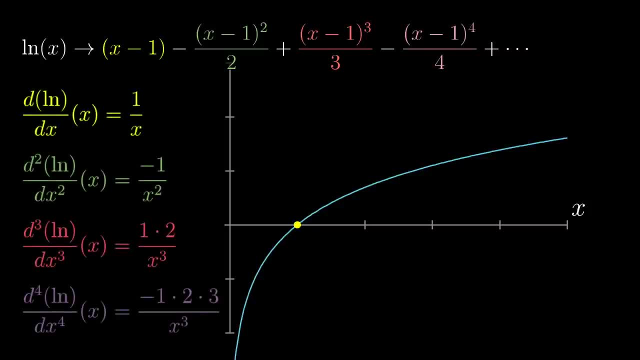 1,, which is built by evaluating the higher order derivatives of the natural log of x at x equals 1,. this is what it would look like When you plug in an input between zero and two. Adding more and more terms of this series will indeed get you closer and closer to the 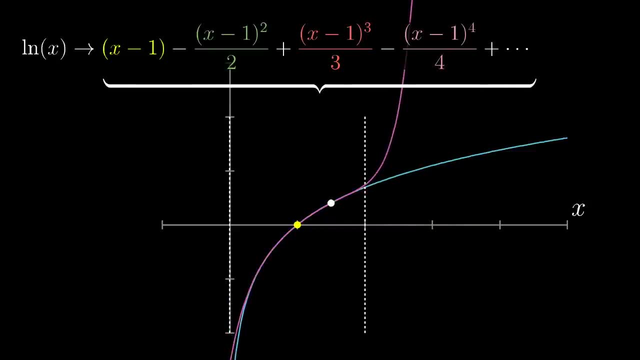 natural log of that input. but outside of that range, even by just a little bit, this series fails to approach anything. As you add on more and more terms, the sum just kind of bounces up back and forth wildly. It does not, as you might expect, approach the natural log of that value, even though 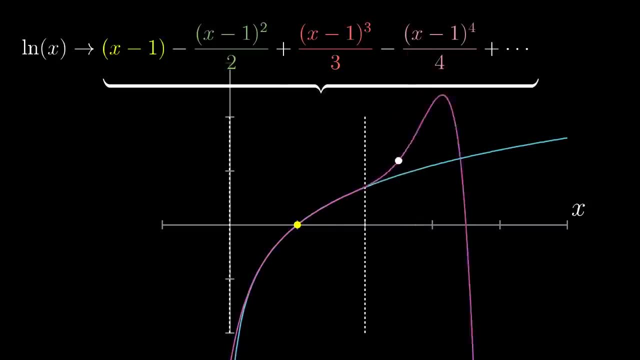 the natural log of x is perfectly well defined for inputs that are above two. In some sense the derivative information of ln at x equals 1 doesn't propagate out that far In a case like this, where adding more terms of the series doesn't approach anything. 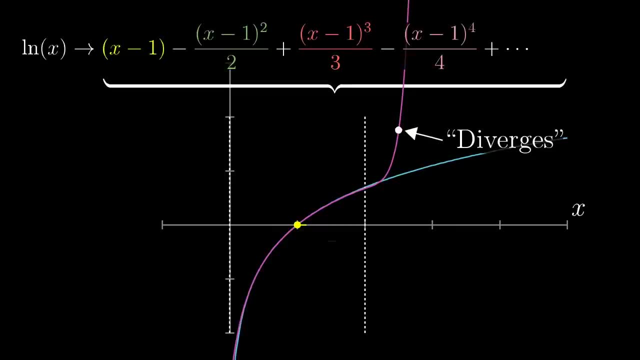 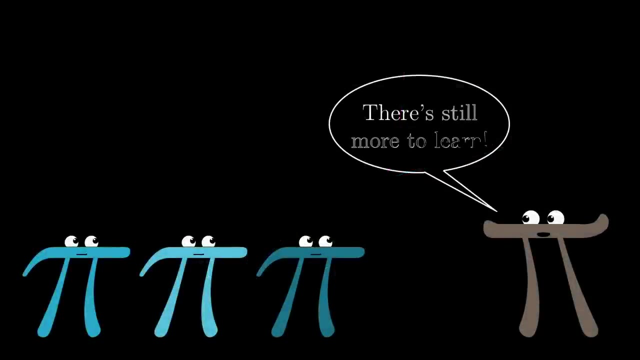 you say that the series diverges And that maximum distance between the input you're approximating near and points where the outputs of these polynomials actually do converge is called the radius of convergence for the Taylor series. There remains more to learn about Taylor series. 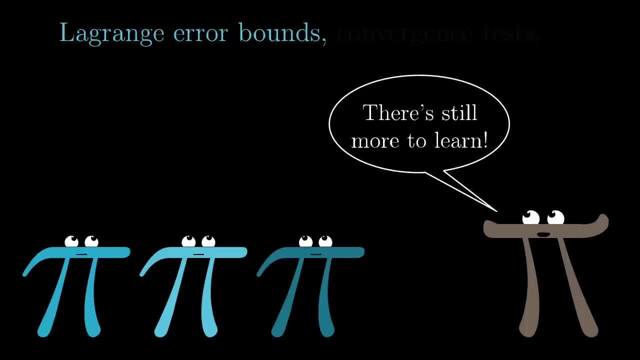 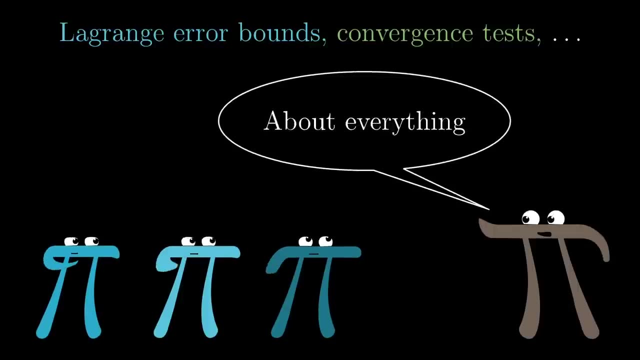 There are many use cases, tactics for placing bounds on the error of these approximations, tests for understanding when series do and don't converge, And, for that matter, there remains more to learn about calculus as a whole and the countless topics not touched by this series. 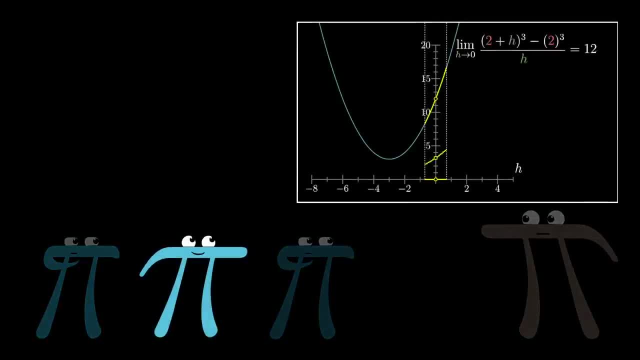 The goal with these videos is to give you the fundamental intuitions that make you feel confident and efficient in learning more on your own and potentially even rediscovering more of the topic for yourself. In the case of Taylor series, the fundamental intuition to keep in mind as you explore more. 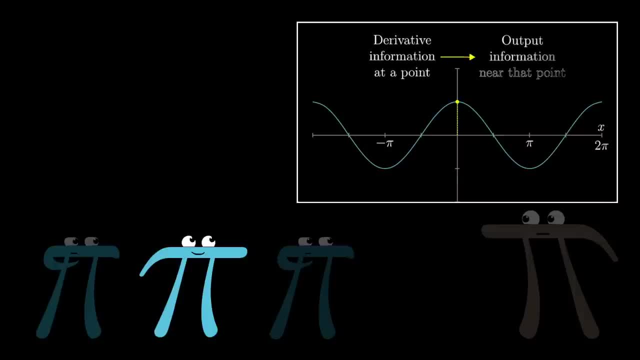 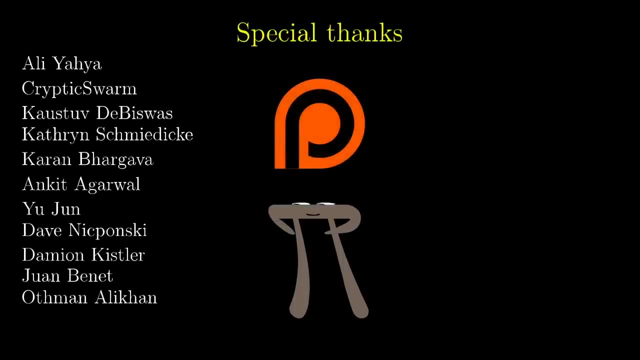 of what there is is that they translate derivative information at a single point to approximation information around that point. Thank you once again to everybody who supported this series. The next series, like it, will be on probability and if you want early access as those videos.